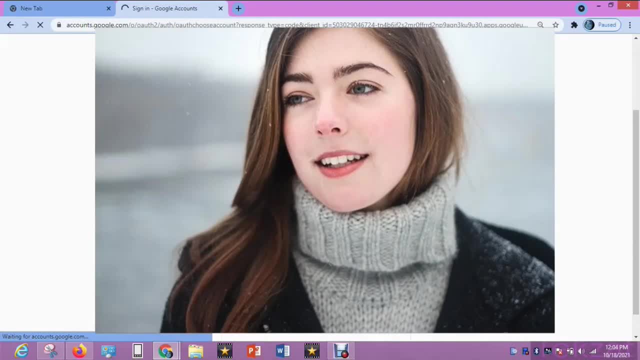 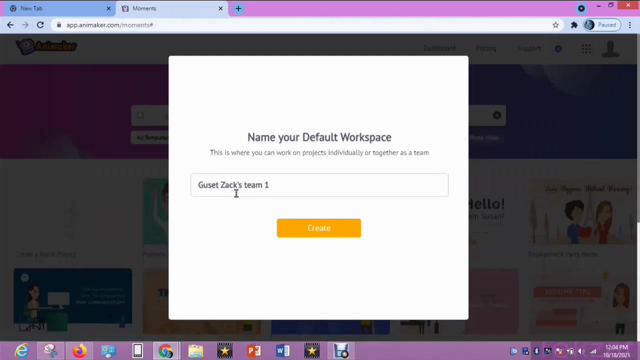 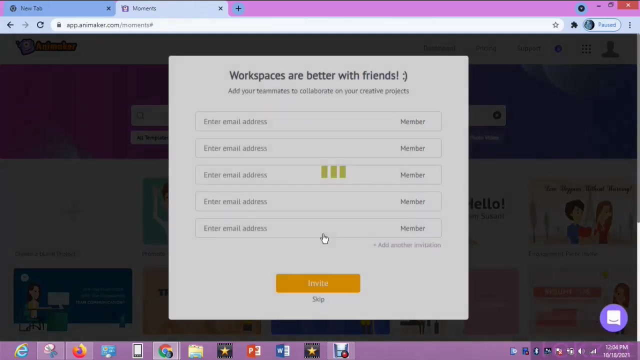 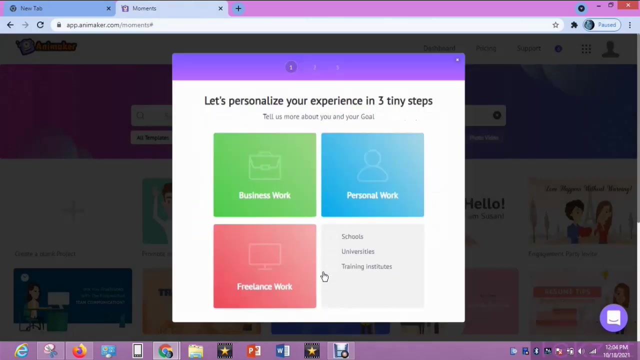 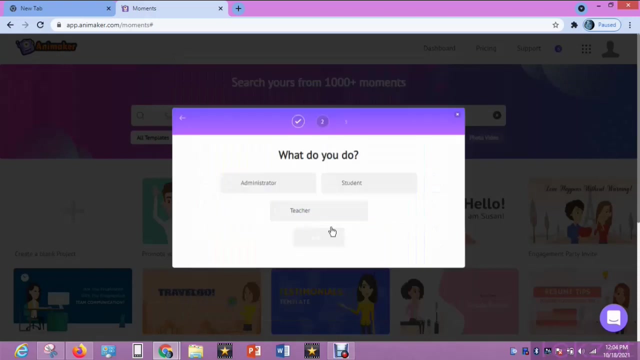 You, You. So I'm going to choose name. use the gmail address name, I'll create new one. I Don't need this. a workspace, a better? No, I skip this. Well, here I went to selected question walk See whether I have some pan for feature. 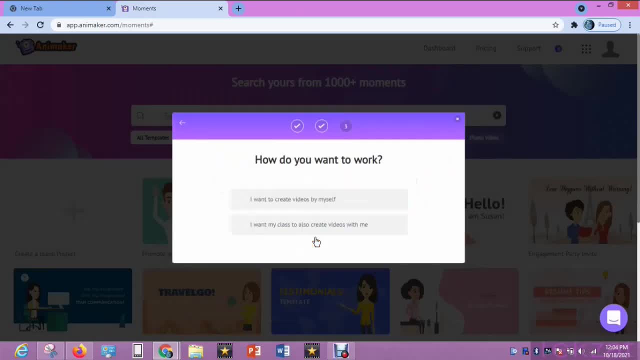 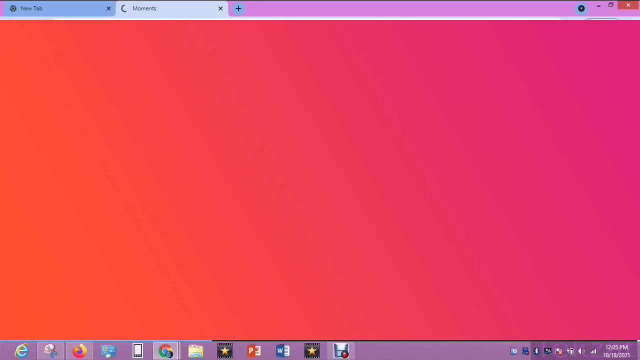 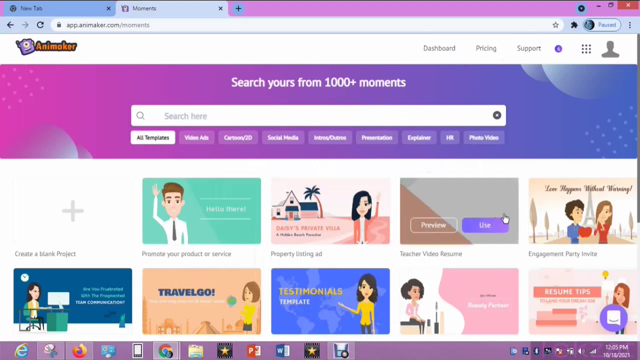 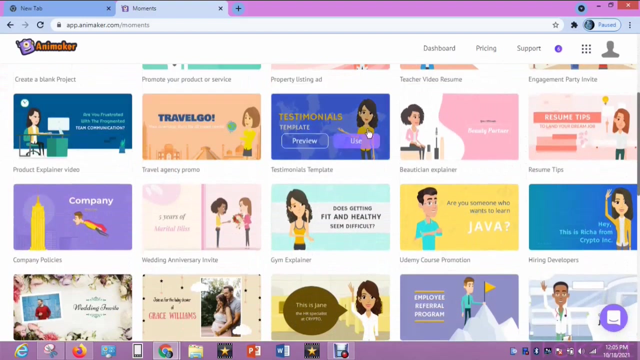 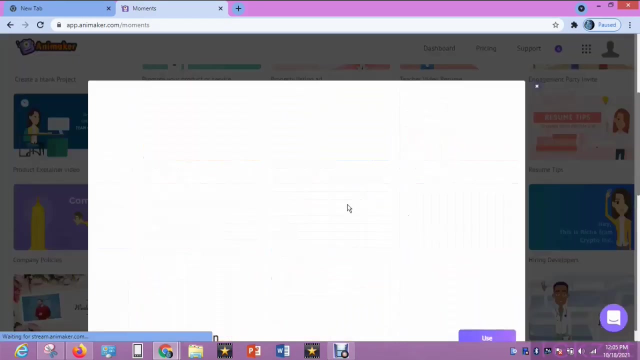 select as a student, then done, So I want to create videos by myself. Thank you for time done. Good, we now have our to anime car main dashboard, not your own personal dashboard. so they already have some clips. they cut templates. some clips already cut template. you go through some of them and preview them and see you can see this one, yeah. 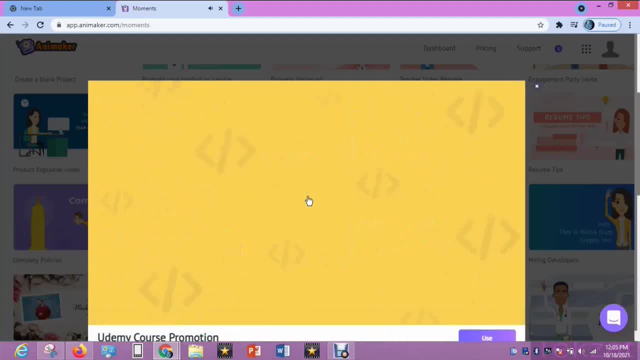 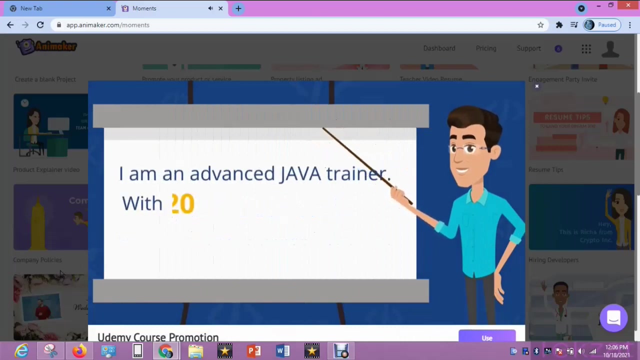 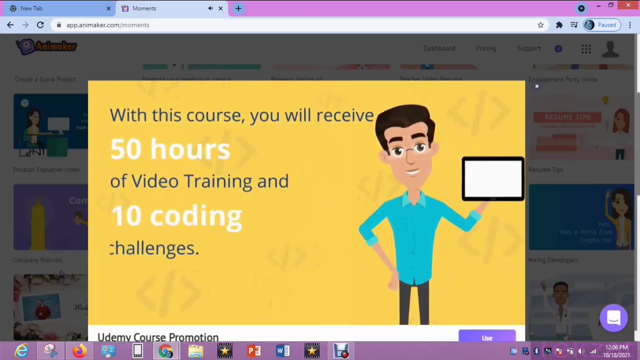 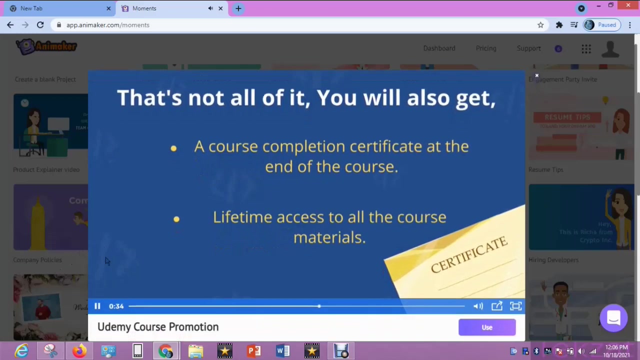 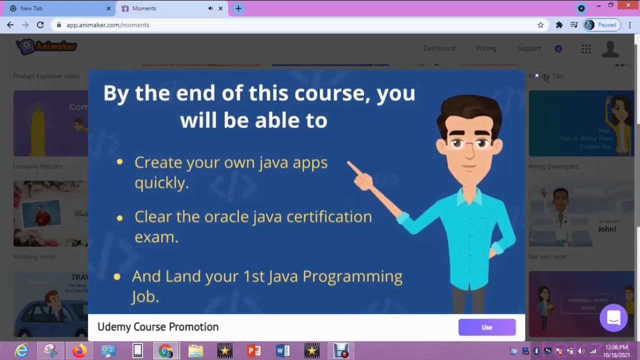 look at it, it's talking about Java. we'll talk about Demi course promo. so you can use this and create what I call course intro. it's nice- or even advertisement. so this is a template. you can make use of it. it's free. what you do is just edit. 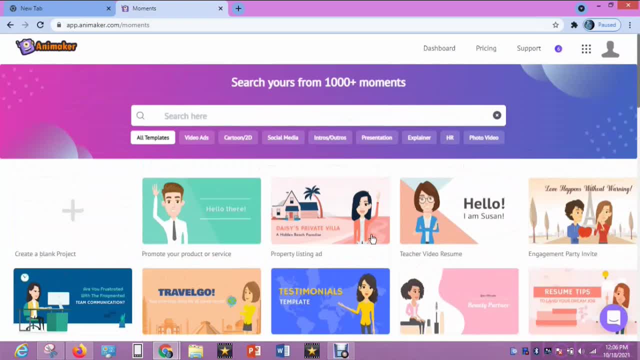 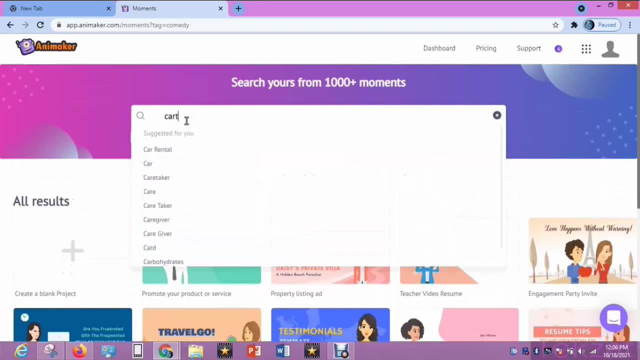 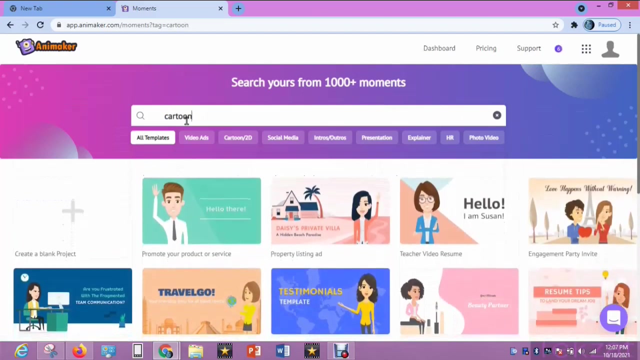 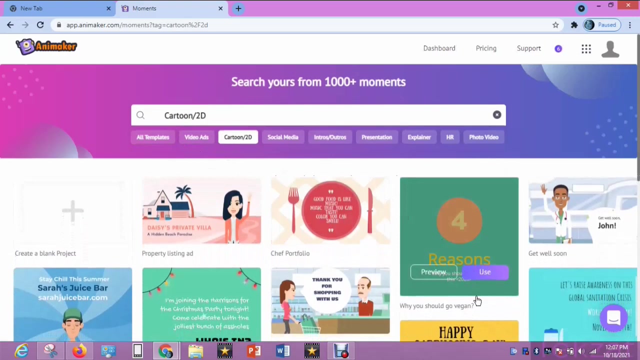 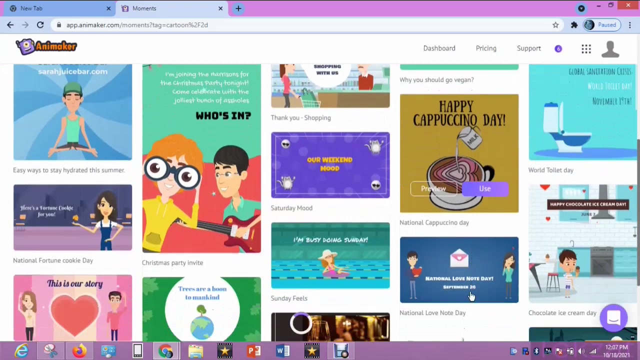 it update. let me search for comedy or cartoon. no comedy. let me search for cartoon. and you, you look at cartoon here, cartoon slash 2d. there are very many of them. we have to go through them. see the one you can use or create one by yourself. but what I'm 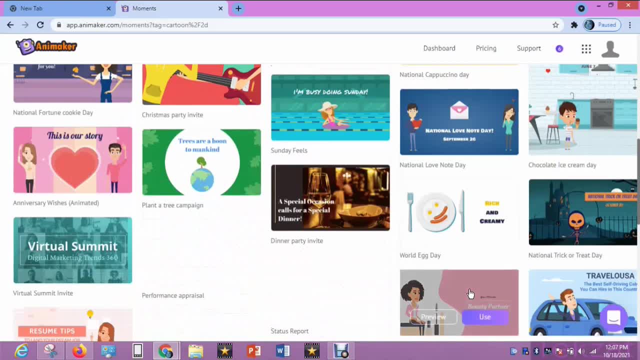 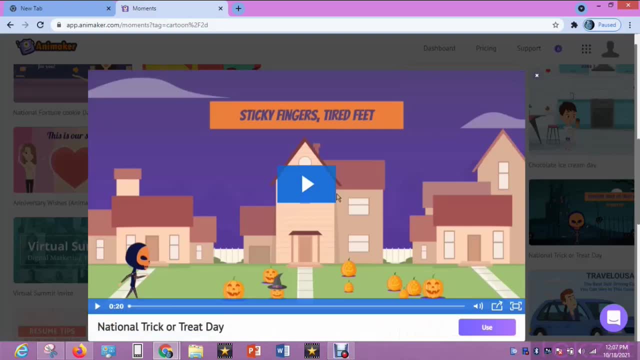 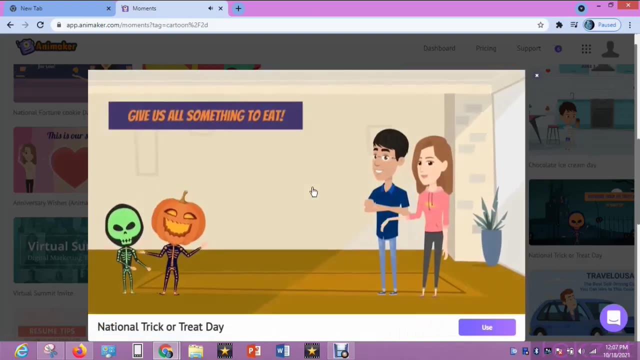 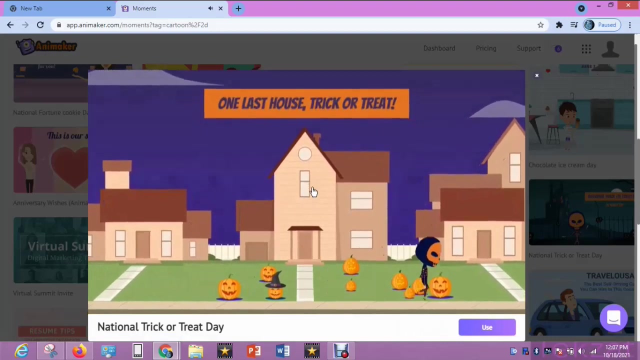 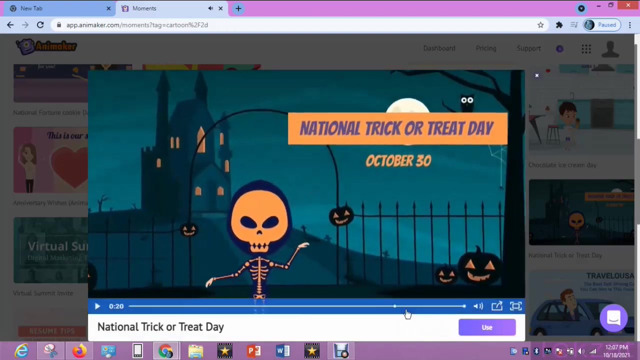 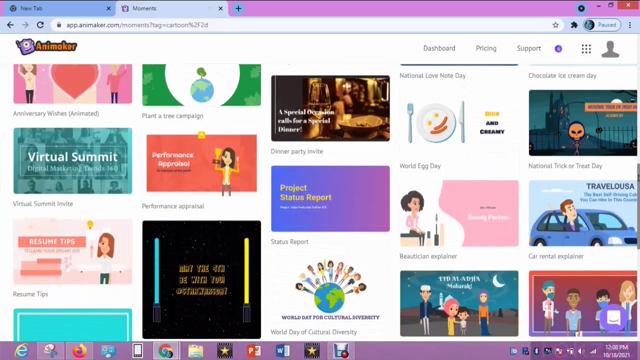 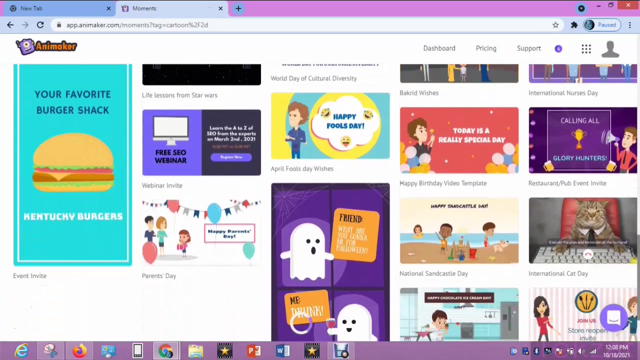 going to walk you through is how you can create a video with anime. come from scratch is a templates. wow, this looks scary man. you can see skirt. think I like a dances, so I can use that if I want. there are so many of them, let's test one or more, preview one or more and see. 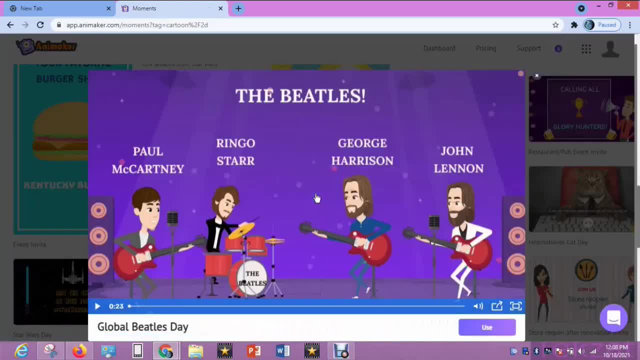 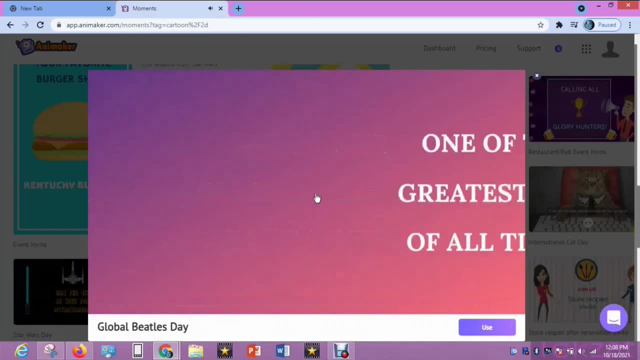 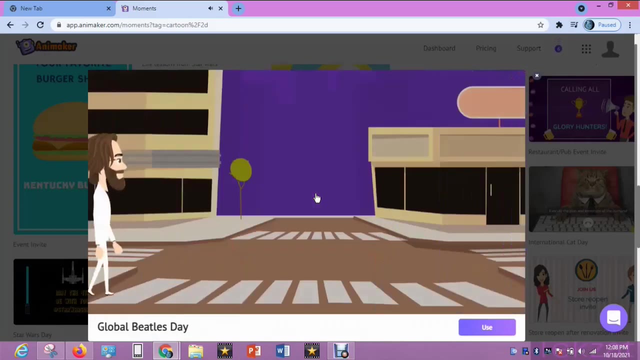 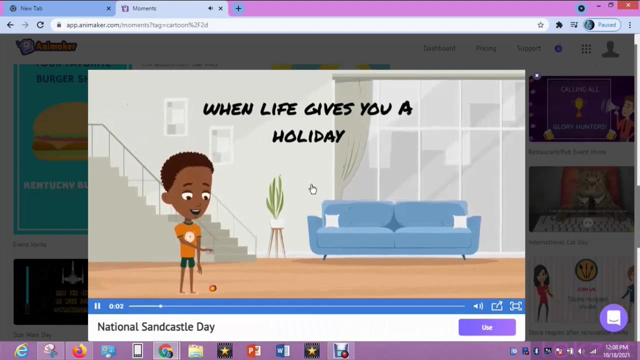 let's come together to help one of the greatest band of all times, the beast. Wow, that's great. man, currently, that's dance, or this guys are going to the club or party. Wow, that's great. love it there like is it. see this one again? Wow, that's fine okay. baby tub. Syria was another cartoon you can see. there are many, that's all I'm comparing the inter operation. every you do this, your full time score, every single video we can see and we've got all the credits of this. refresh me al text on that che� call her. 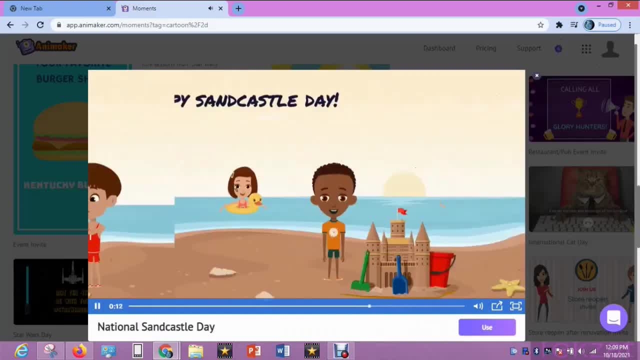 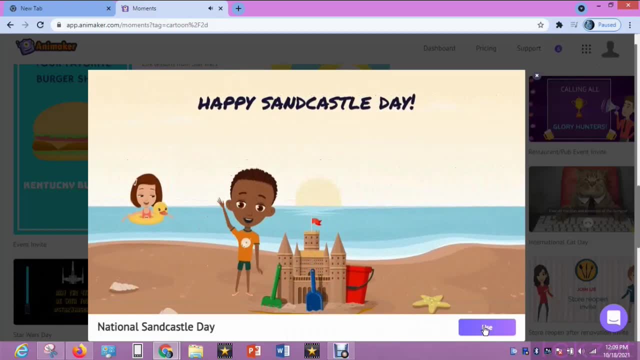 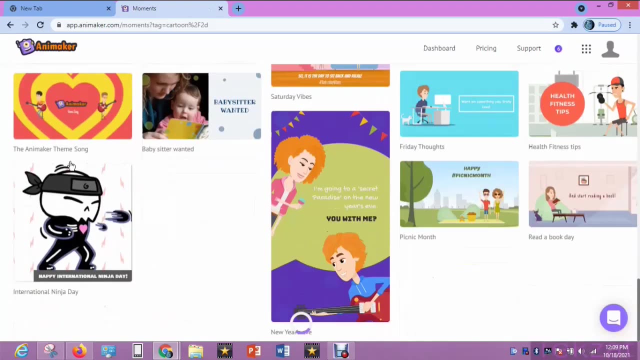 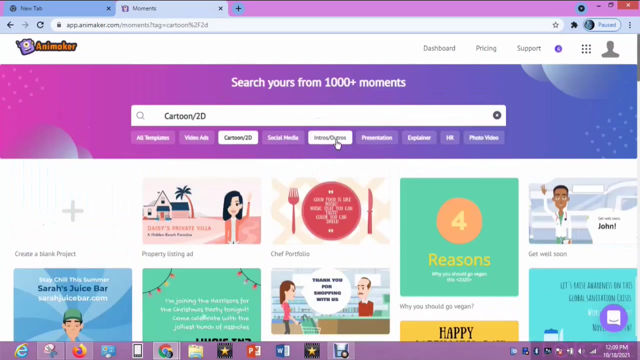 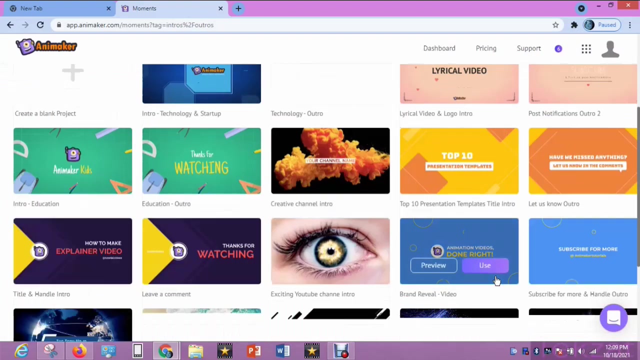 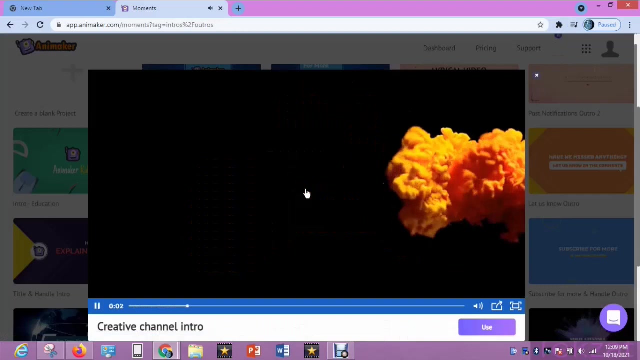 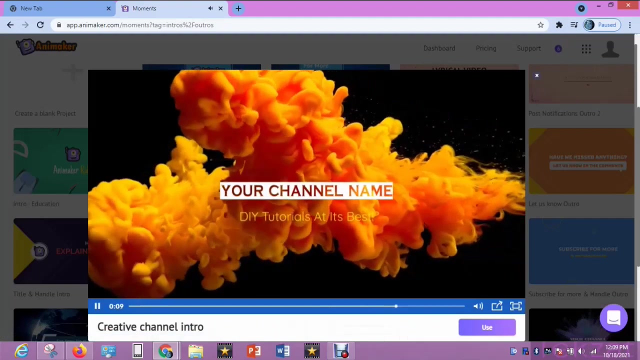 or tingolo and now maybe encore twinkling. okay, can use it as well and do the necessary. it now more and more. but now start our business. can check out that once nine through. you can use where YouTube channel you may have one. this one is nice, the nice intro. use that, or remember, if you're not using paid plan, that might. 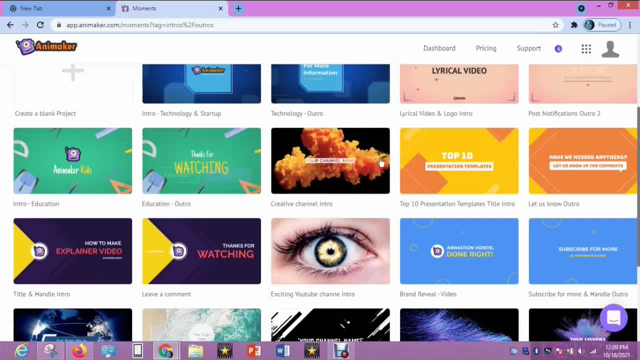 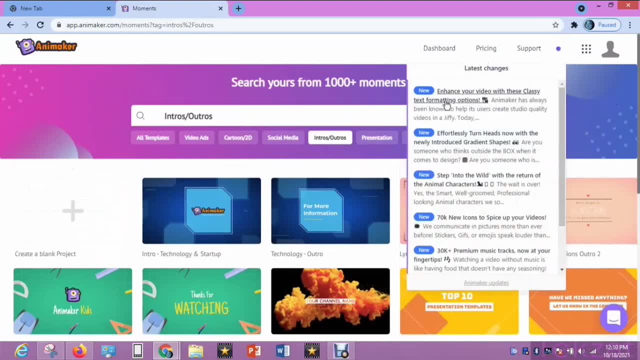 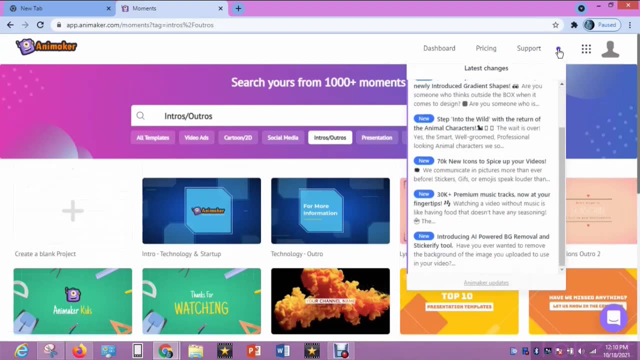 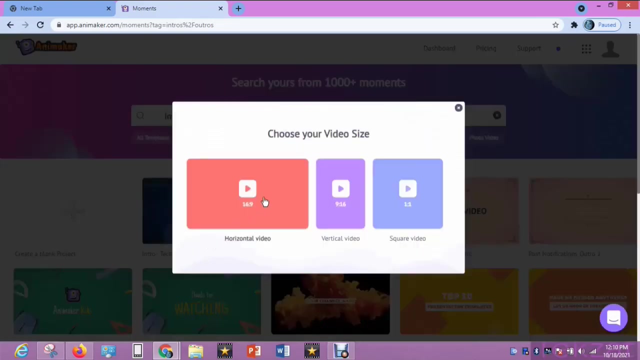 be a watermark. there must be a watermark, not maybe. so that is that. let's see the message. okay, good thing about a new maker. good, so now let's create a project. we're going to create blank project. now, three different landscape. use here this particular. I can use it for YouTube shots as a vertical video. it's an ID for. 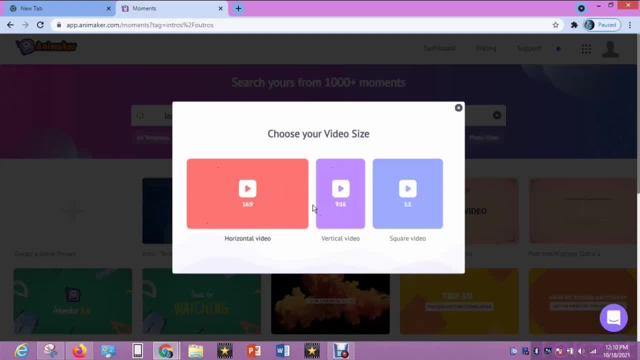 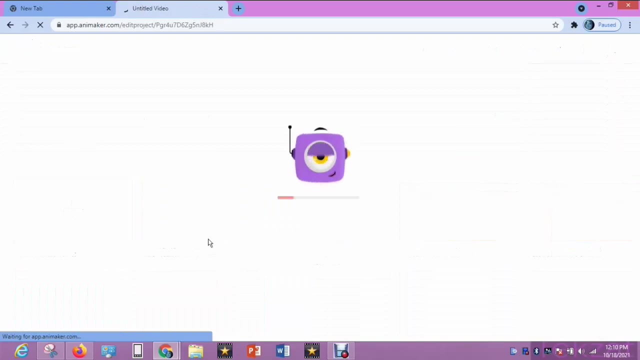 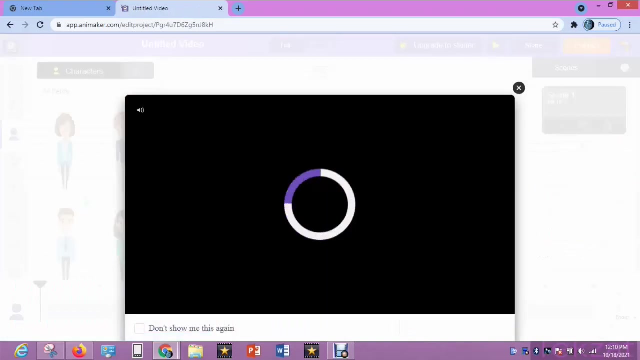 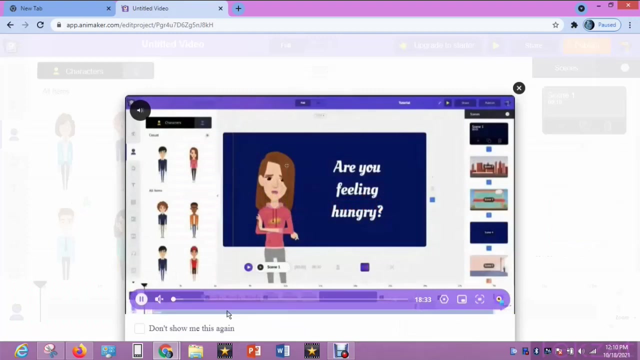 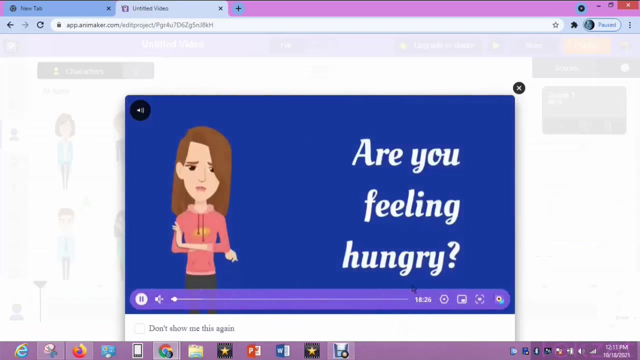 YouTube shot. I start then this horizontal video. now what are going to create? they do square video, so let's create a horizontal video. and my car is preparing our worksheet and other things. yeah, say, watch a video. you're telling you I can make use of it. this guy looks all sad man. okay, is there some of the car? 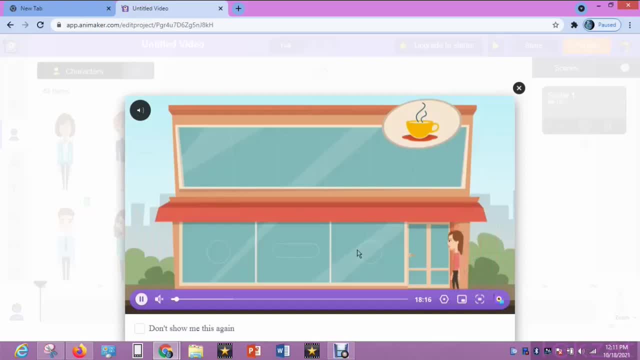 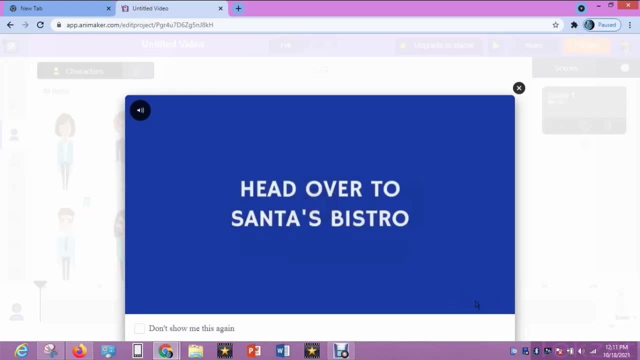 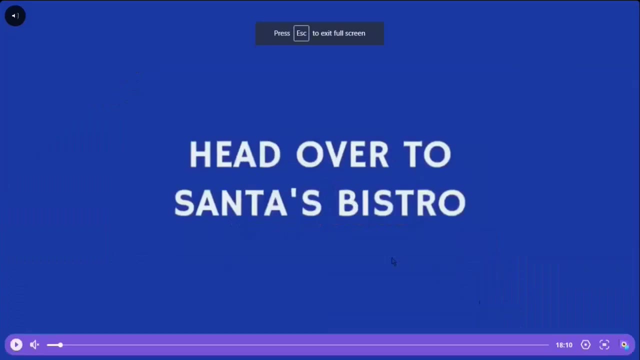 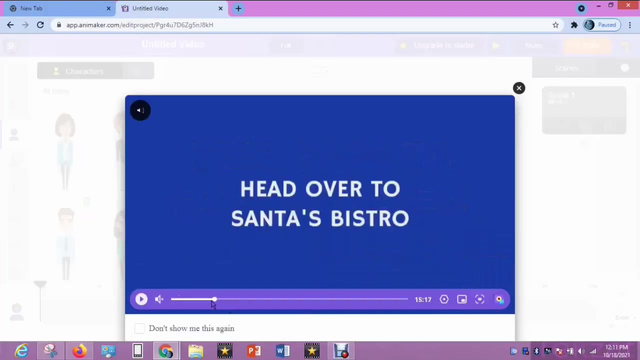 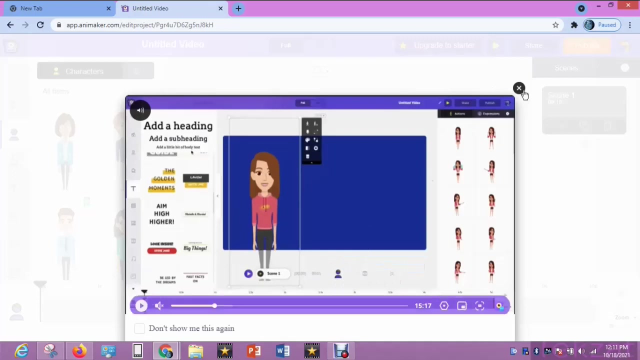 authors, background image and other things. that's when I spun that. okay, dishonest passion. say head over to some past Bristol, please throw. you're showing the example, same way we see on templates, but here is telling you how to make use of it so you can see a new. please ensure you watch the video to the end, so get ready you. 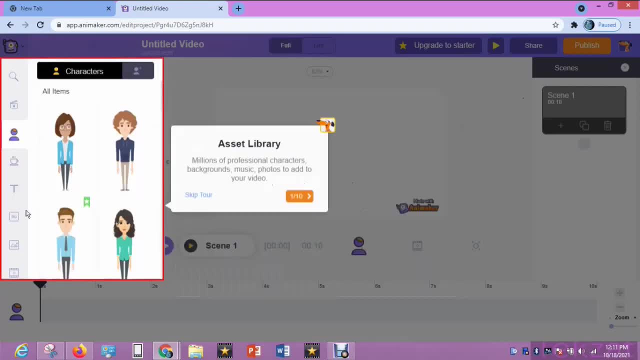 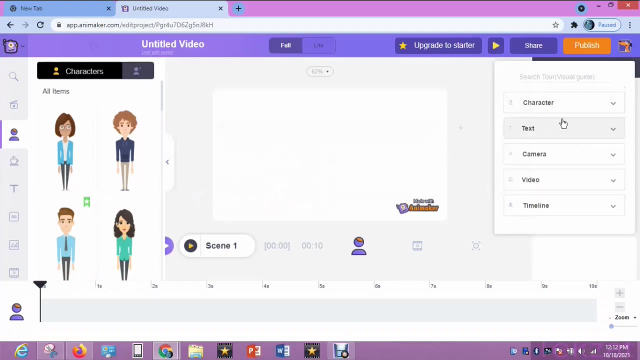 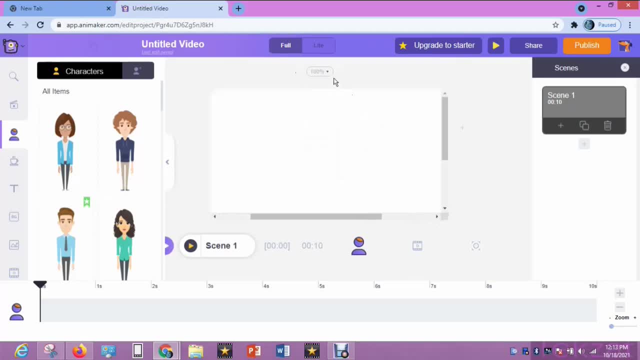 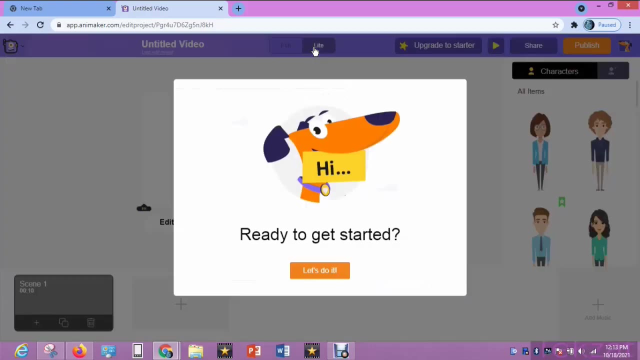 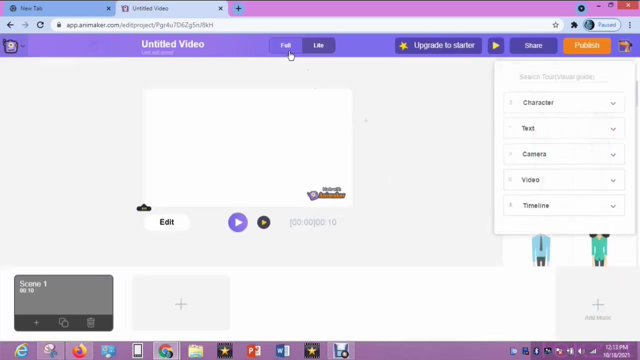 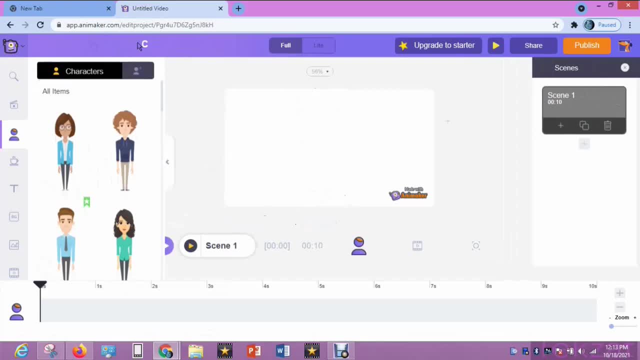 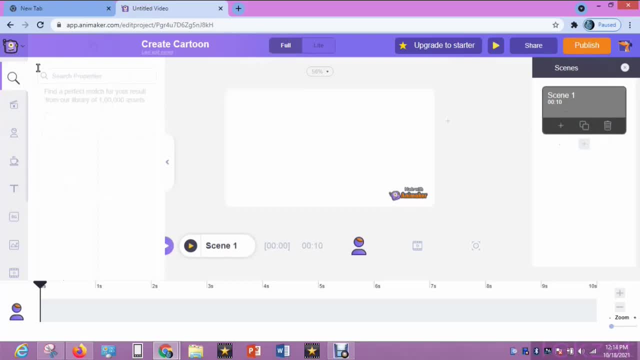 anything from here, anything you want that's available on the resources, you can get it from here. let's start for landscape. this is a landscape. most of them are paid. anyone you see with that green icon is paid. let's start for something like background. good, most of them are paid. also, let's look for okay. 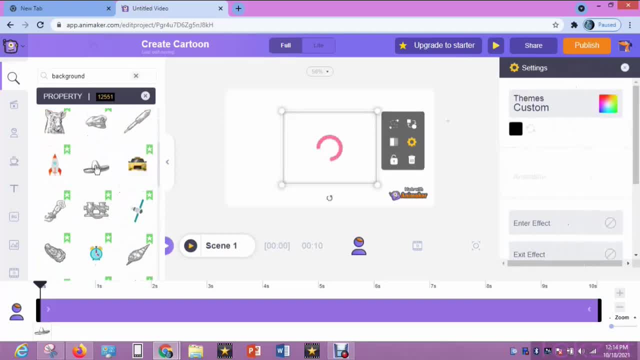 this one is not paid, doesn't have a green icon. good, it's. a background can change the color. there are many options here where you can pick from. you can drag it to any position you want. there, we can change it here. let the beauty of it turn it upside down left. 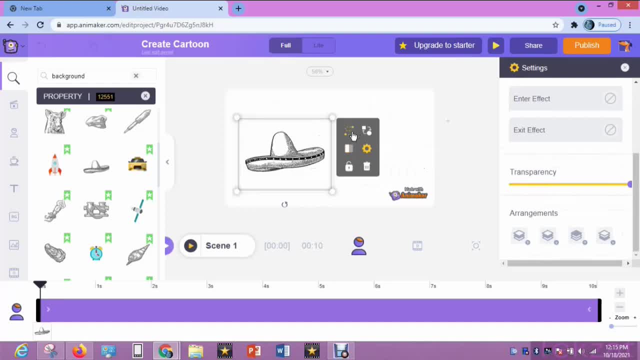 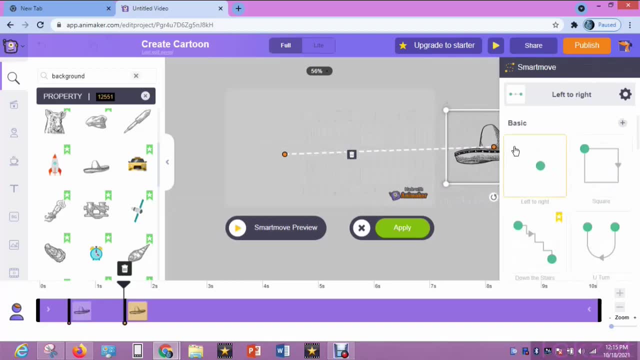 and right. you can make it move from here. I can move now. drag it to a new position where to move to. you can drag it to a new position where to move to. drag it to a new position where to move to then test smartphone preview as you can see it here. 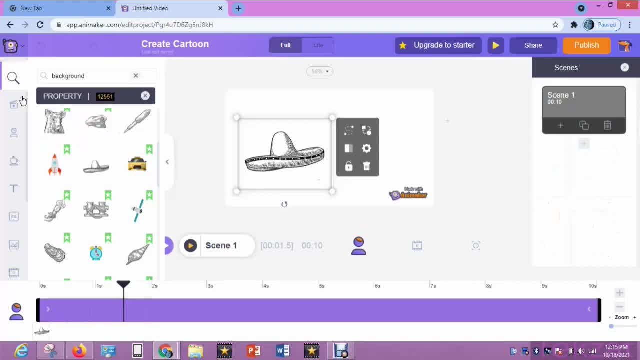 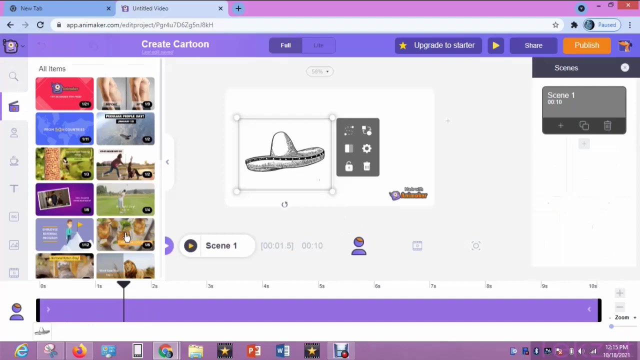 mean animaker has a lot of features which you like. so go to video. this preview template, just like the ones i've seen before, you can see many of them, anyone you pick here. there must be another watermark because i'm using free plan, but if i'm using spade plan you will not see what i want. 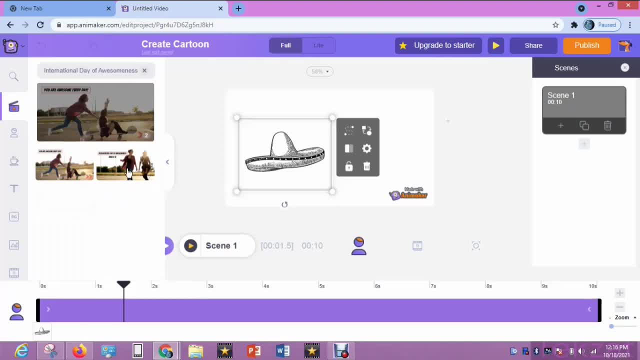 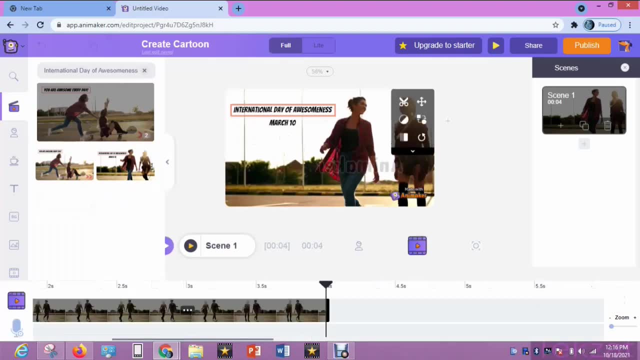 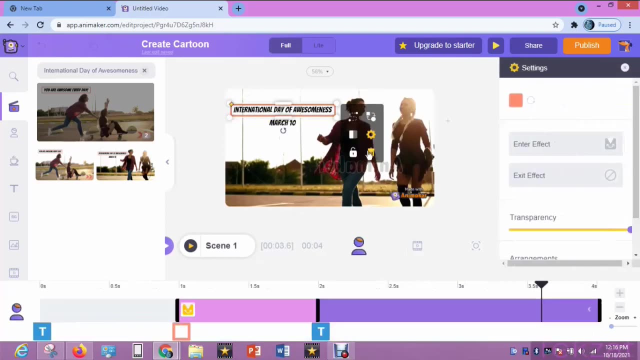 like this one. you can add it. it is when you are adding, depending on your network. you have to wait a little because use this network to upload and it takes time. like if you want to publish this video, it takes a lot of time, no matter how small it is. so this is an example of a template. 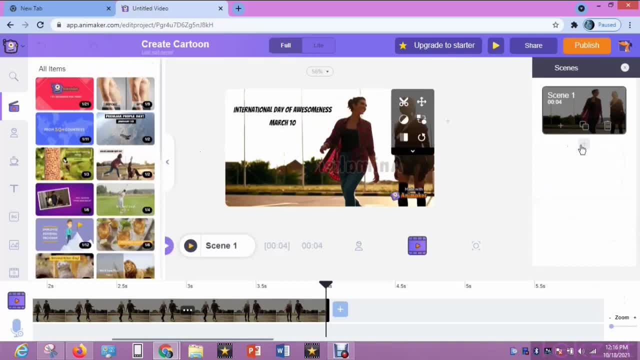 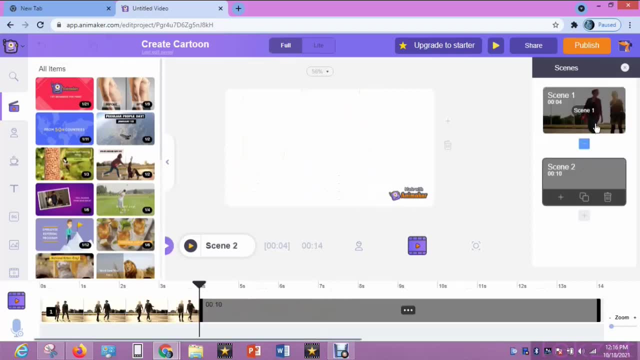 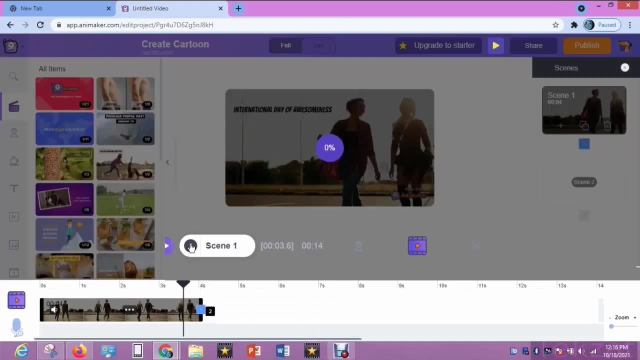 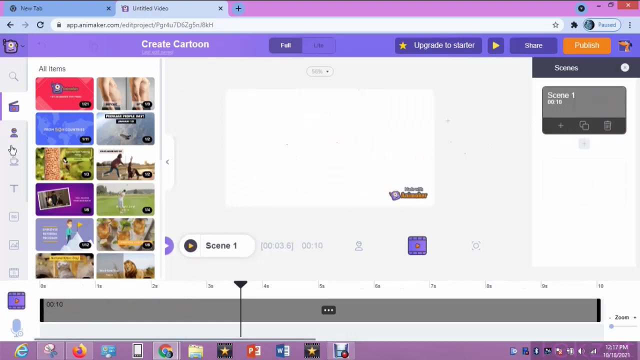 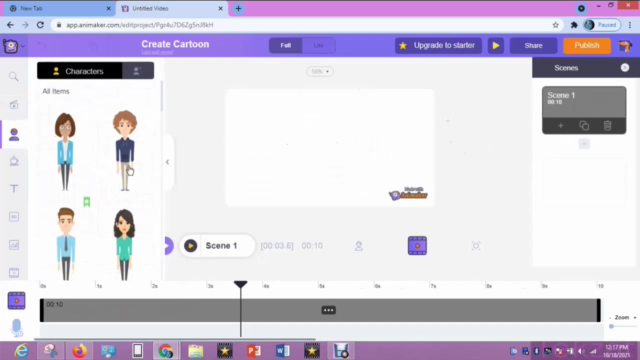 can edit it and whatever i want to do, add another scene. i've seen two. when you click on that play button, give it some time to load. good, this is my characters. this is the main thing i'm going to work on. you can see, we add one. 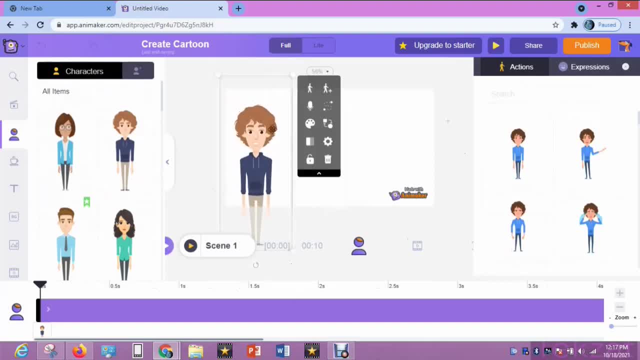 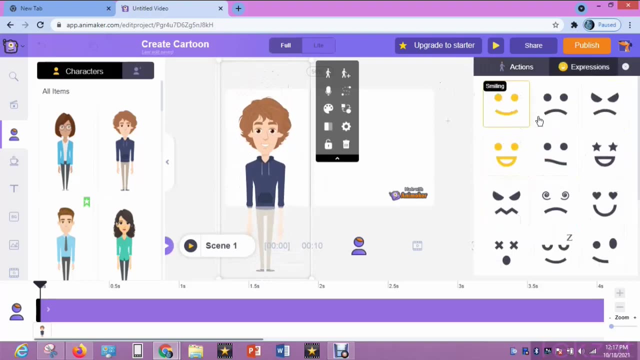 can either increase the size or reduce the size, depending what you are working on. if you are working on a presentation, increase the size. very well, like people will see it, i can change the face: happy mood, sad mood, wow this, there's love in the air. here. there's love in the air. 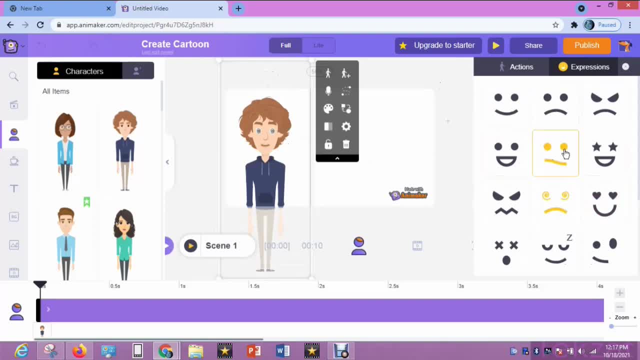 let me change it again. that is cool. the guy is um annoyed. let's try once more. let's look at this one. what the guy is angry here, so let me pump action to it. standing with anger, with angry face. oh bad man. oh you can't see, wow. 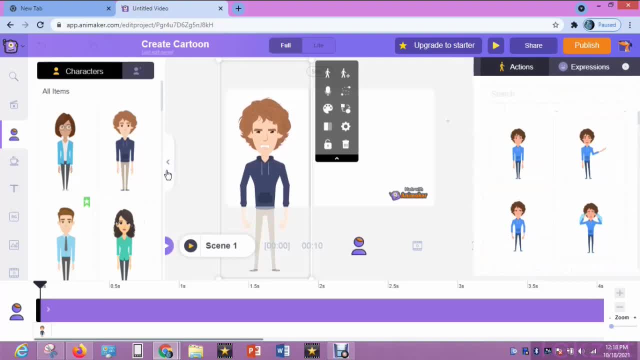 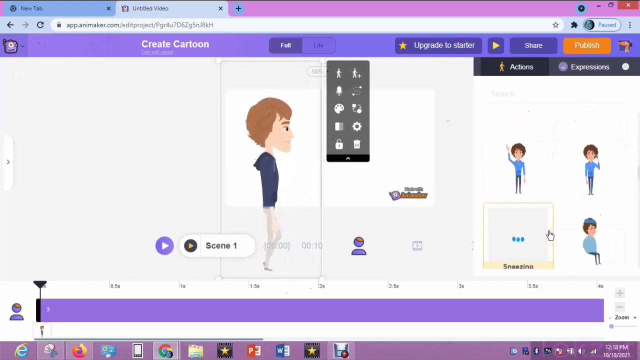 yes, angry man, he's just angry. so just an example. there's another example you are going to see. yeah, anyone you choose from your right hand side, this particular character will turn to it as we choose: walking. you can see it is now working. you can reduce the size. check all actions using pc: sleeping. 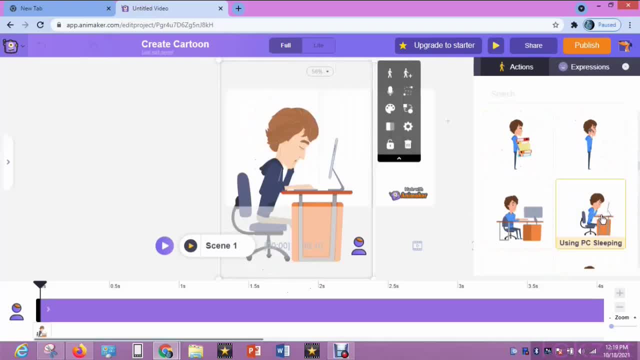 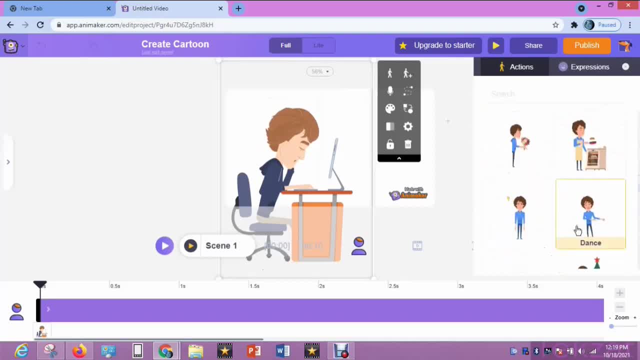 so i'm going to change the size of the character. well, it's dancing here. let's see, yeah, the cool guy is dancing. that's fine. wow, just dancing, let's dance, dance, dance, okay. well, there are a lot of features in anime car so we can change the speed or change the time. 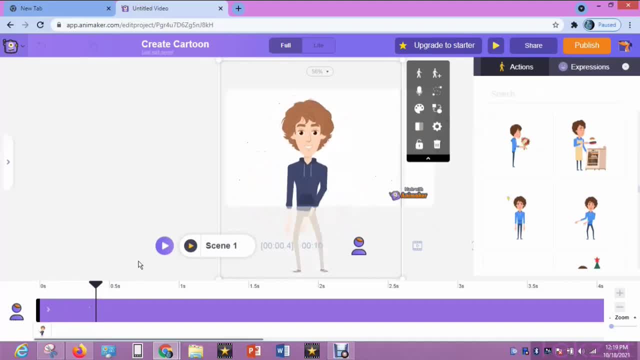 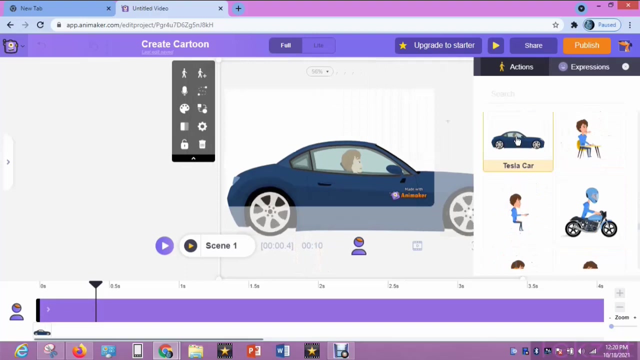 there is a character sb, some particular action, there's other actions for this action taking place. we can control the time, understood the movement and other things. search more. could i just see a car? okay, that's locked car. wow, it's great, this is great. can you see that? can you just beat that maybe? um. 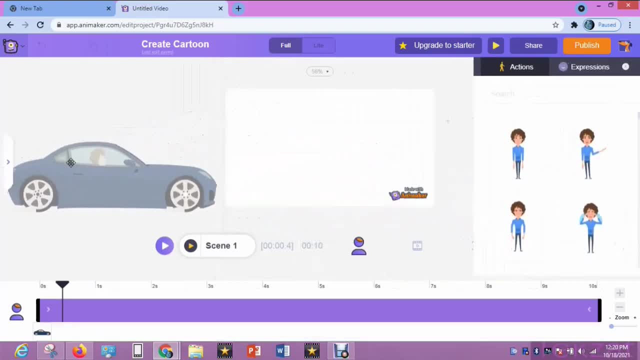 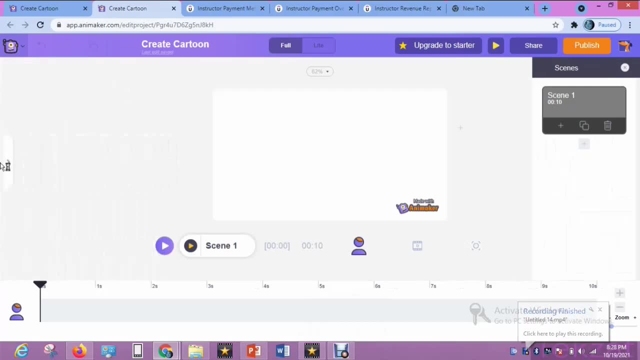 that wonko is driving pass, so let's drive it pass. choose the part and then let's use our old background. we'll click here, go to background, then we'll click here, but that will not allow us use our own background. what to do is scroll down from here. 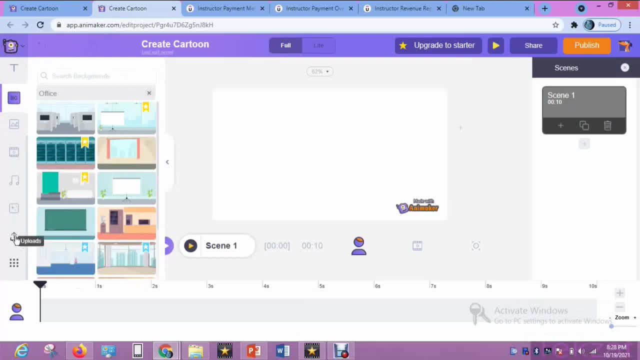 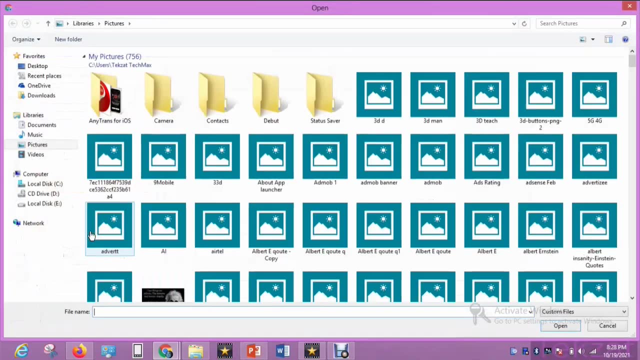 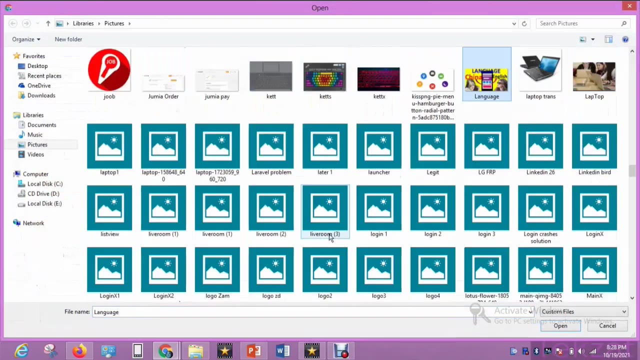 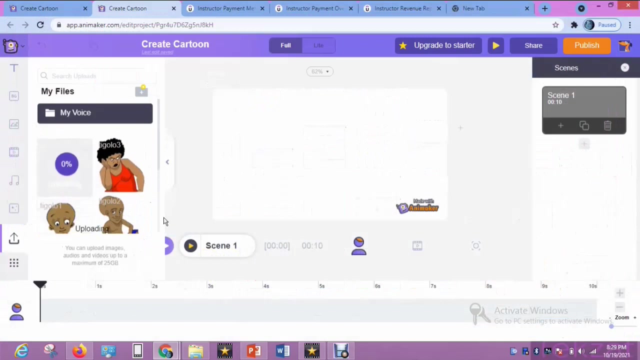 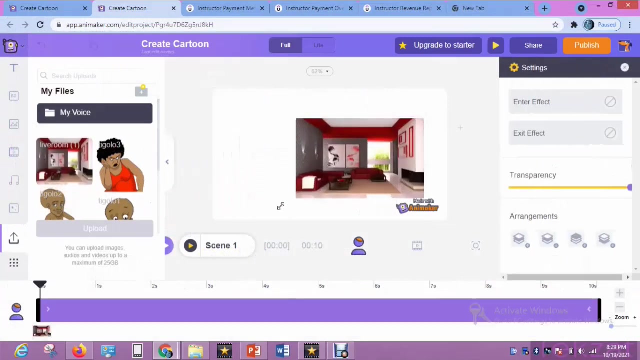 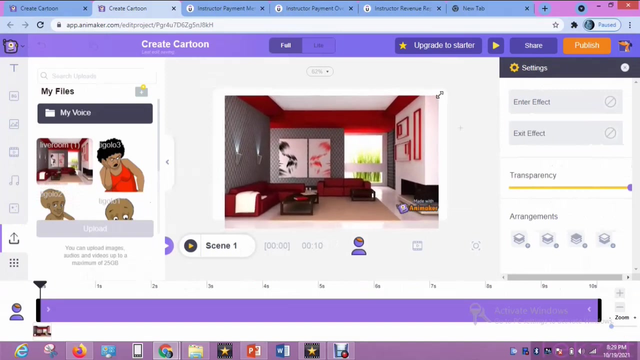 click on this sign. this sign means uploads. then we'll click here. i already have my background. it's living room. i like to upload finish. sometimes there is a little bit slow so i drag it to my workspace and the next thing i will increase the size is a nice living room. 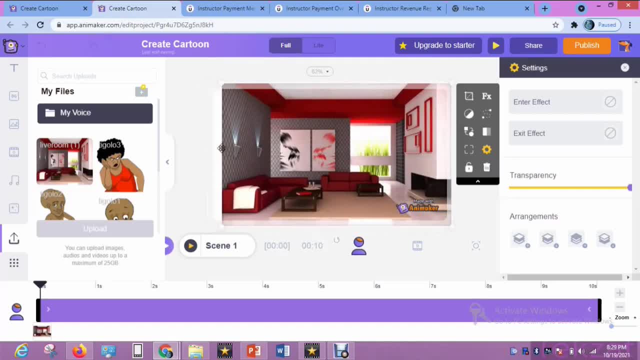 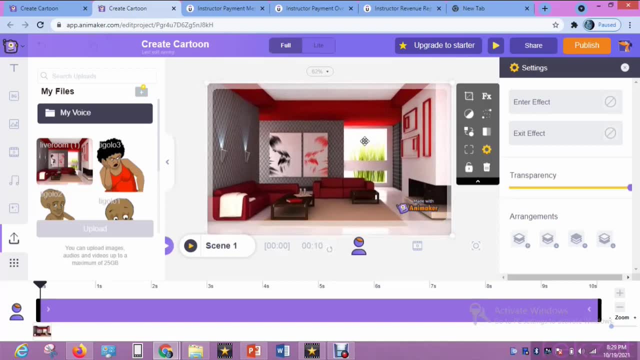 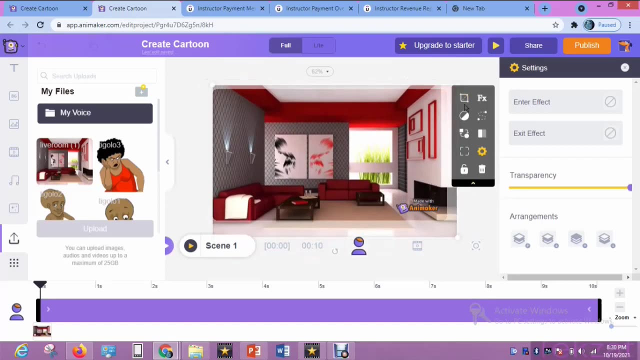 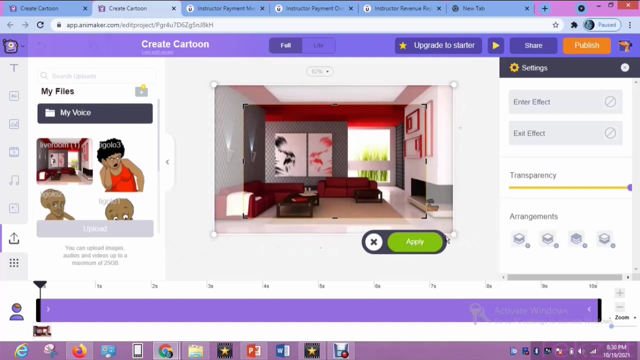 make sure to cover the workspace, like this area that is white. you can see there. we're going to check from here. it is size. let's try and cover the workspace. uh, there's the workspace. check here too. this is the workspace. so it's my workspace. this is my workspace. 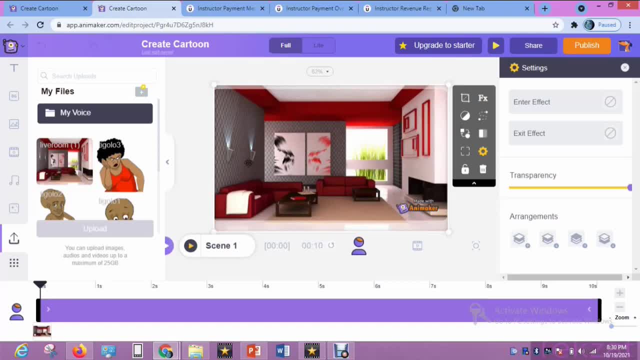 oh, that's fine, i'll apply that. so the next thing: i've uploaded my image the same way i uploaded this one. so i'll bring my martingale. this is my martingale. i'll reduce her size, do her size again and to put time as you end. 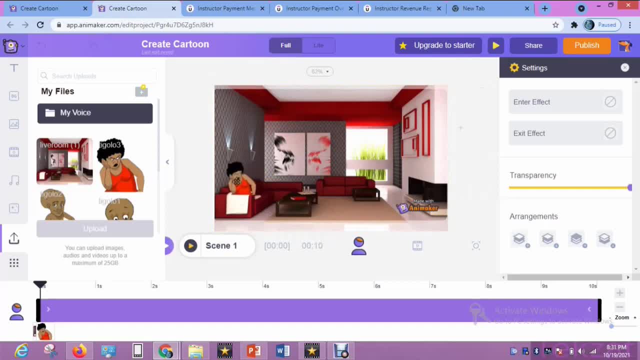 i'll put here here, as you can be here, and then you can see. it's supposed to have legs here, all that things. so what we're going to do now is we're going to cover a little bit space so you won't see her full body. cover some space here. 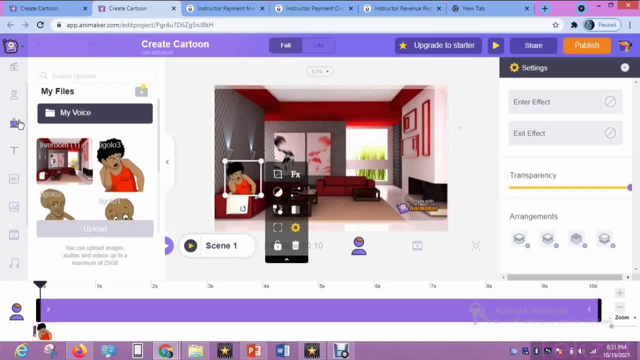 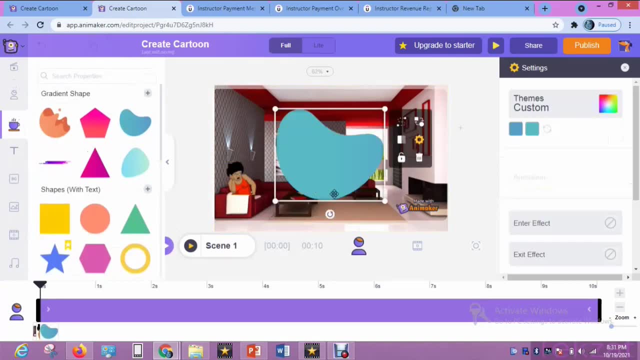 so go here, roll up, click on this, tick up. all right, let's use this guy. yeah, so i'll reduce this side. first of all, we change the color to another color will look like our setting. something like this will be okay. that's gradient. reduce the image. when i reduce the image and keep it here you can see. 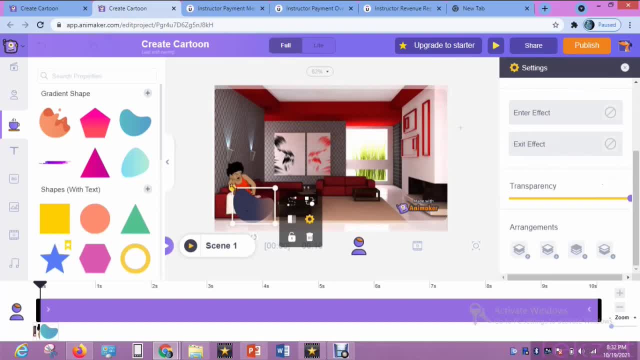 so here's a cover. martin colo. okay, good, remember just practicing something and with time you'll be perfect. yeah, so, like this is okay. well, let's find another one, let's look for another one. let's cushion this self. well, i'm gonna use this guy. 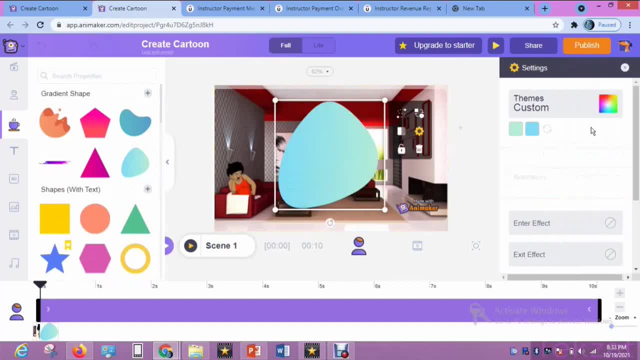 so good, i'll remove this one and use this one. let's change the color. let's change the color. we'll remove this color. i'll change you what i don't really know. i say no effect, where's it go? i'm going to use this color. i think that's fine a little bit, and then 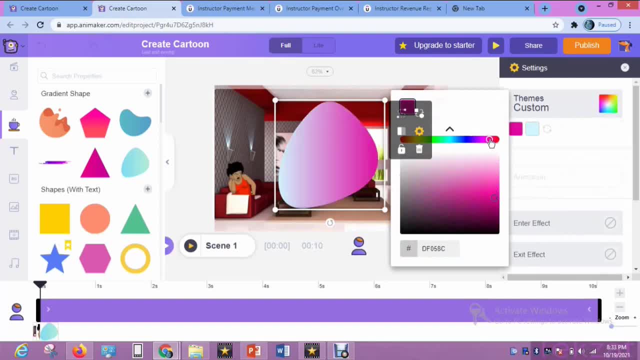 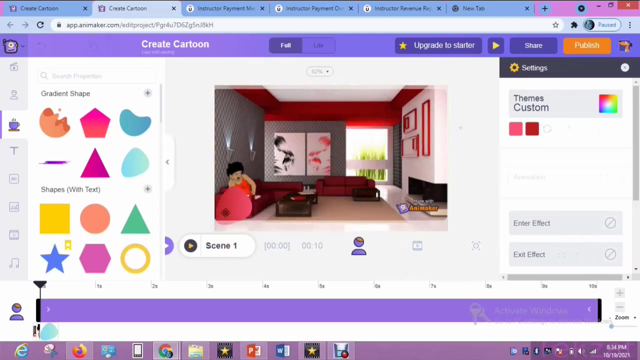 let's go, let's go, okay. okay, It's a gradient, so be careful when you're working with the color. Wow, Okay, Yep, Thank you, That's the color of the room. I'll reduce the size and push it this way. 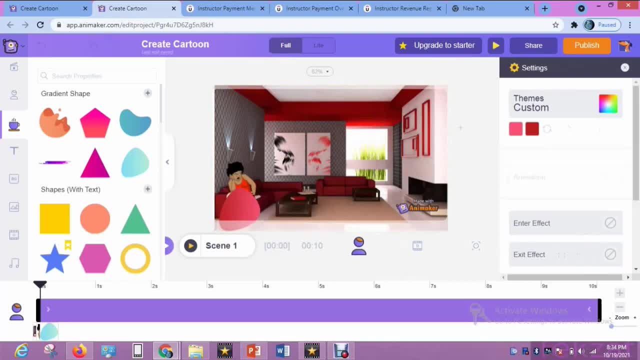 I'll expand this more. Hold on, I don't know what I want. Come, Okay, This is okay. You won't know that she's not there. Okay, Okay, Okay, Okay, Bring in our select. So the next thing we're going to do: bring in another image. 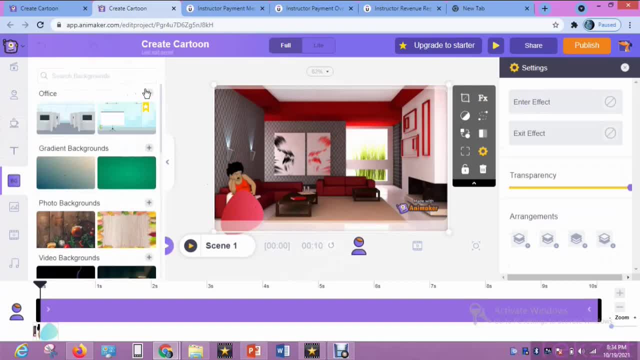 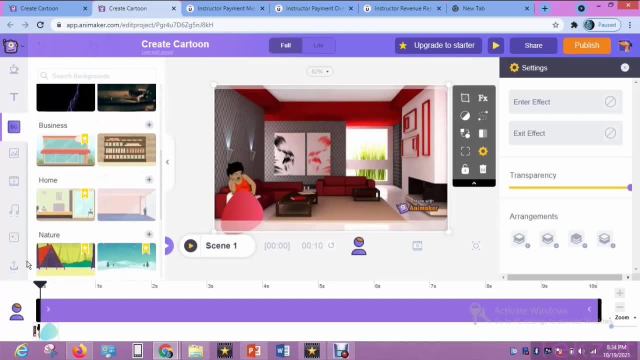 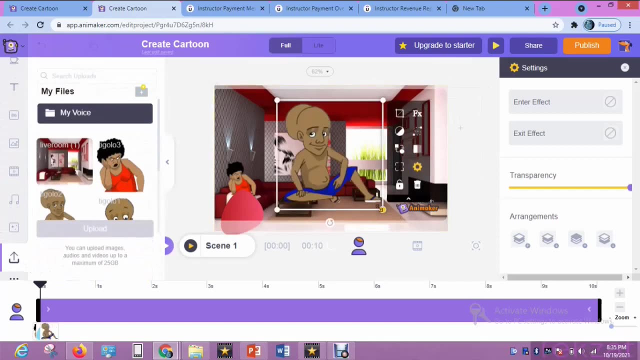 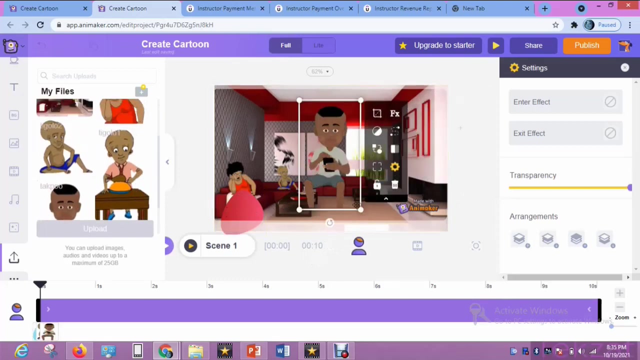 I'll stay working on the image. Go upload, Scroll down, Go to Upload And bring thing. Oh, Oh, Everything, go low, little aside, the big boy can relax somewhere there. so gradually building our room, we are on the wow, finally, this table, the top book on me, here is a table. 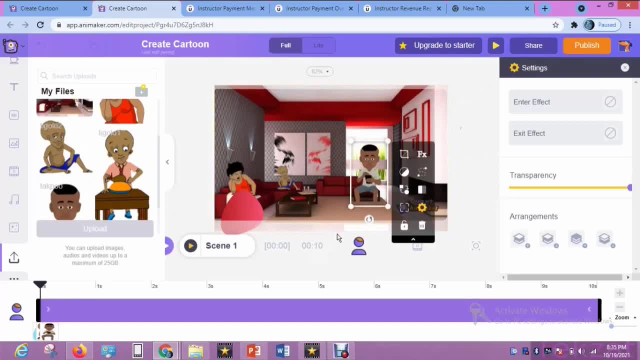 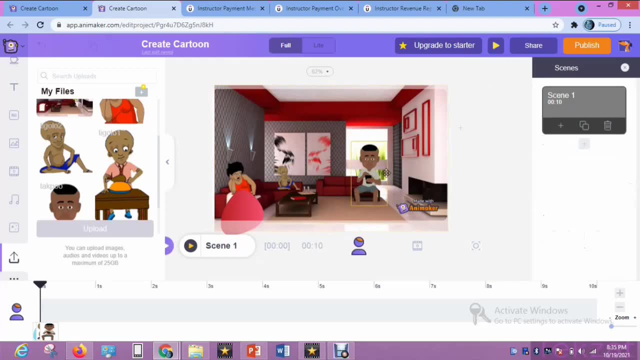 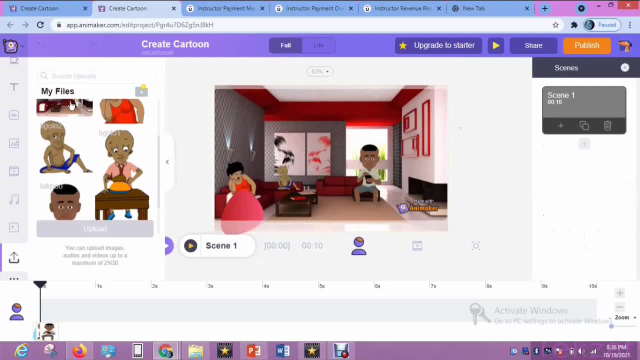 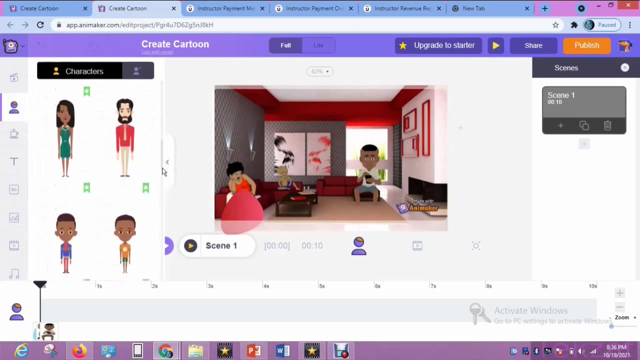 it. I'm working on it. ah hello, my house adding some вос では找- investigate. now let's find a Sur dramaあ, I'll look around them best to find which one I'm going to have a start there, there and now is a closed door. that. 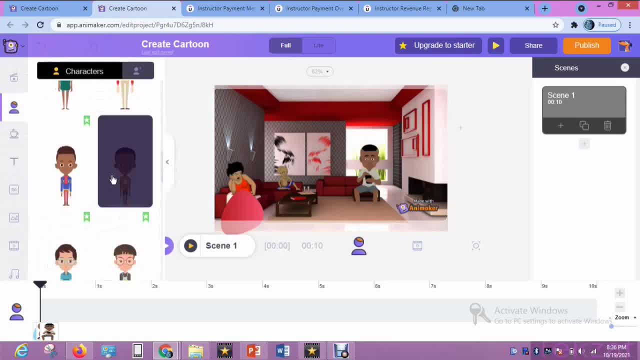 I'm not really opening it. see if I can find the door open. So this guy is happy, he is in a spot because he just peed. I know This is um Karata Rokyo. Okay, I'm not going to choose anyone for now, because the next I'll show you how to be the Karata. 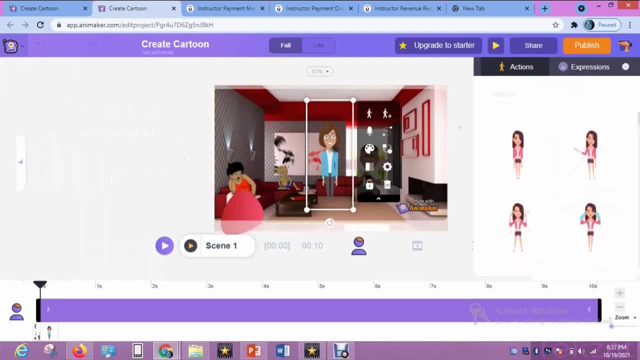 I'm going to choose this guy and then we'll go outside. it's going to enter, Go to work, Okay, Okay. Well then the next thing, I'm going to smart move. I'll draw the path it's going to follow. 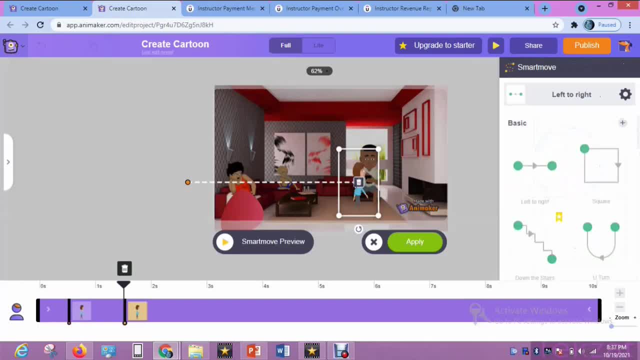 So click here. You can see it comes here. So I don't really want to, I don't. Good, Once we come here, let's reduce the timeline. This should take at least 2 seconds. 2 and a half seconds would be ok. 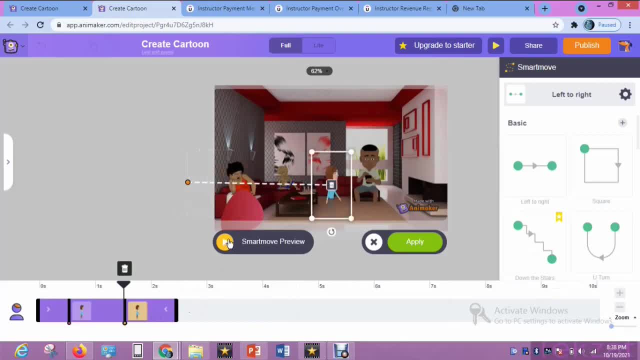 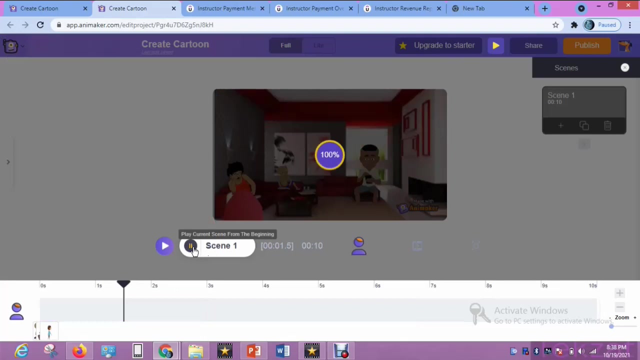 Let's watch it A little bit faster. no, 3 seconds would be ok. ok, we are going to apply that. no, let's see it, Go. Let's see it again, go. Let's see it again, go. 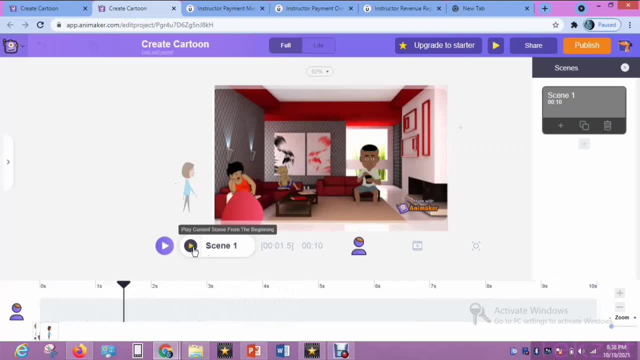 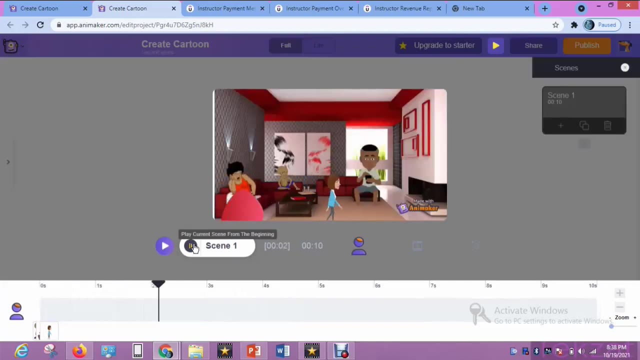 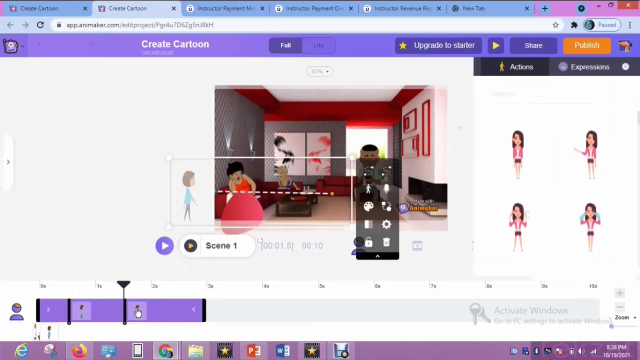 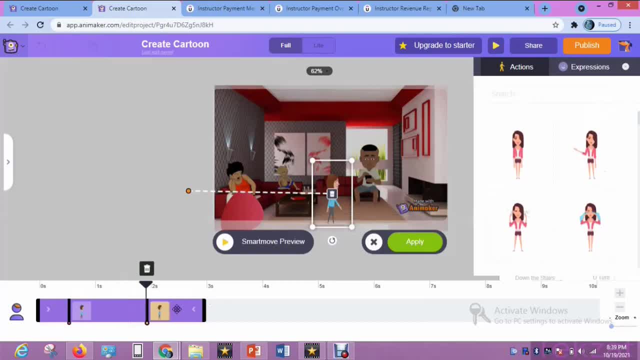 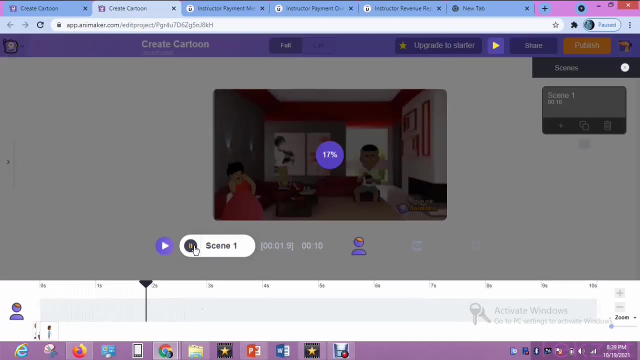 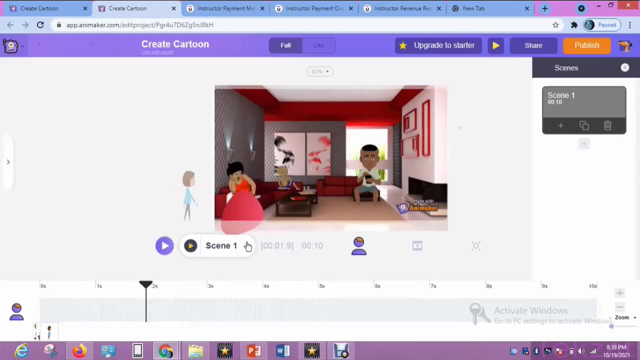 drag it a little bit and now one little cut it off. so let's see, Ok, well, that's it. so I'm going to release this as I hope. 6 seconds, so this guy will now come. I'm going to bring another one in clock here. I'm going to bring that in again. 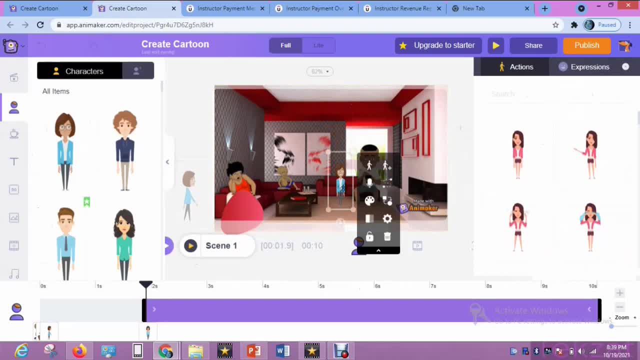 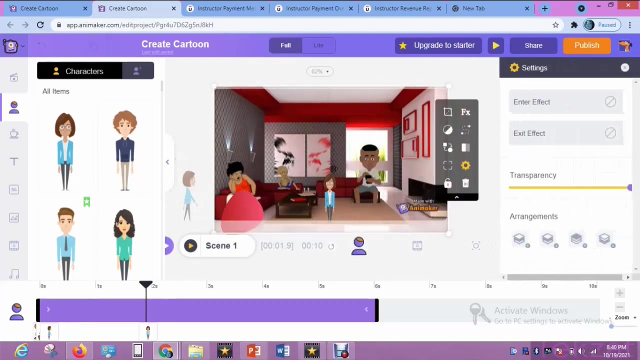 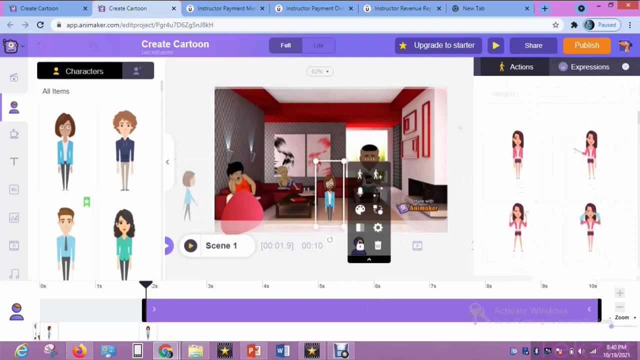 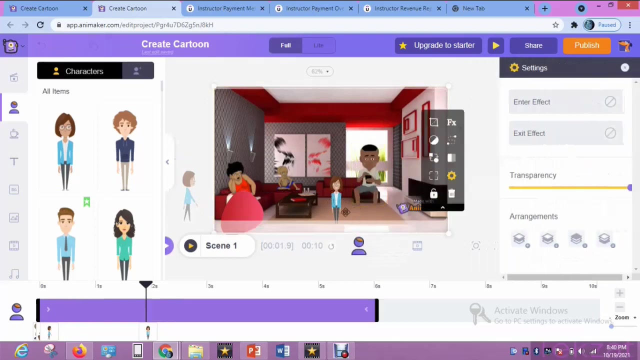 I'm going to reduce the size. make sure the size is the same thing with this one. so bring it over here, ok, ok, yeah, that's cool. So get where this one stops. Stop somewhere here. ok, move it a little bit. wow, now, I've seen this guy will now. 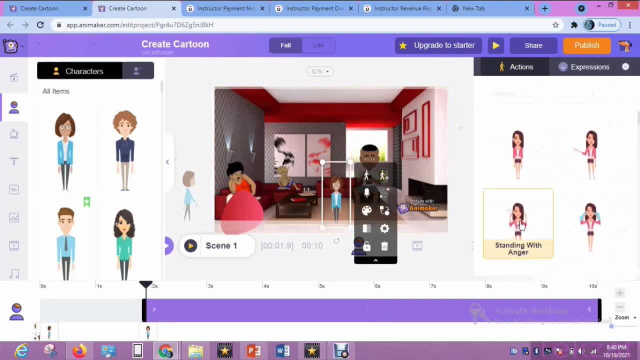 talk. Let me stand. which angle? no, yeah, I'll stand here standing and talking. yeah, so there is this guy. remember this one stopped at 2.4 seconds. yeah, 2.3 seconds, ok now. 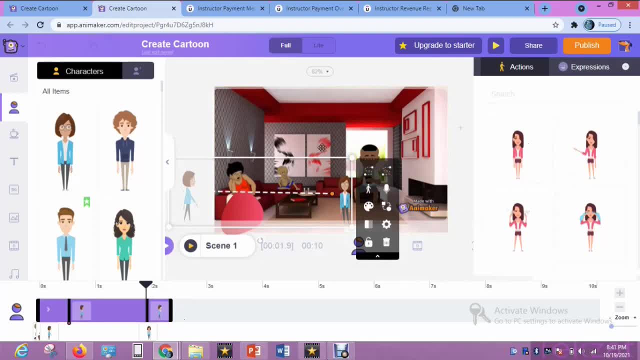 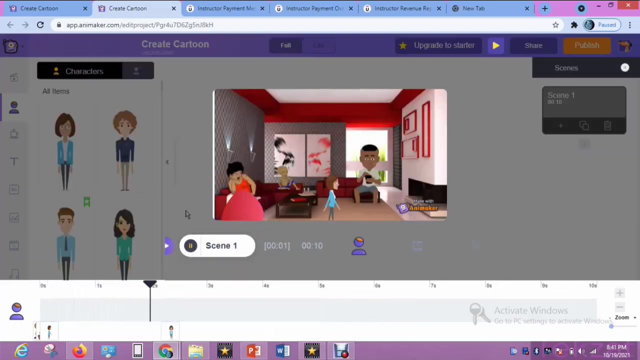 this one here will start at 2.3 seconds- good- and stop at 5, good. that's good. so let's preview it and see Good, So, yeah, Ok, Ok, Ok, Ok, Ok. 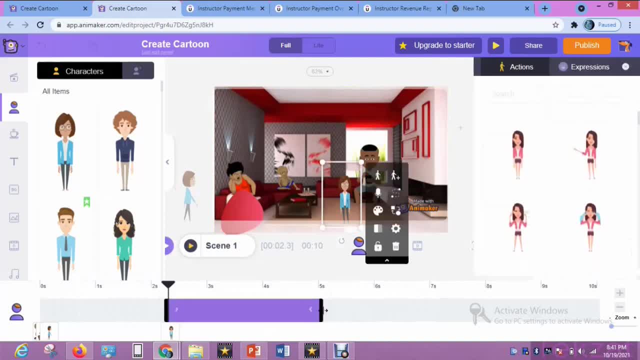 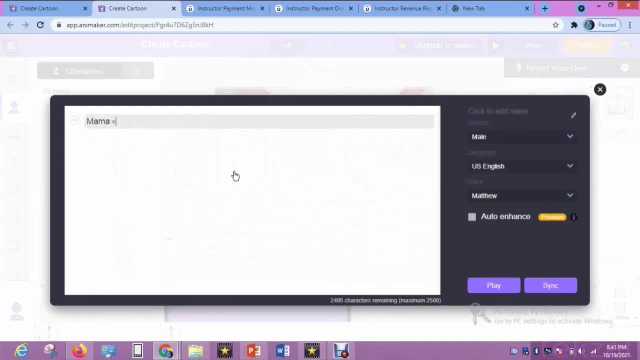 let's see mm Make the stroke here to down, kicked back. so mm make the stroke here to down. so mm benefits Mama tingolo, Mama tingolo. let's see this one say mama tingoluo. 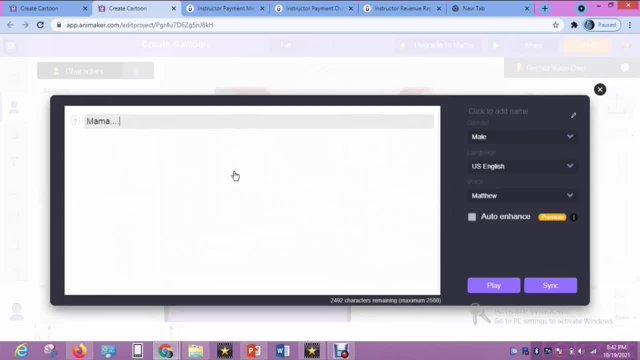 Mama tingoluo. Mama tingoluo, she did the push-up. single 1,2,3,4, 1,2,3,4 comma. 1,2,3,4, single 1,2,3,4. 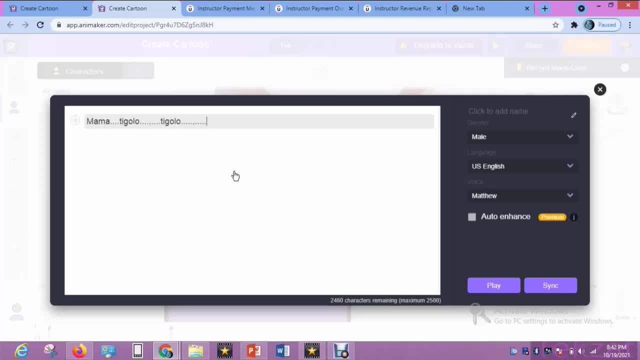 double: 1,2,3,4, 1,2,3,4, 1,2,3,4 set. 1,2,3,4 is wa, So let's try it. You change this to female And we're going to use English. You. 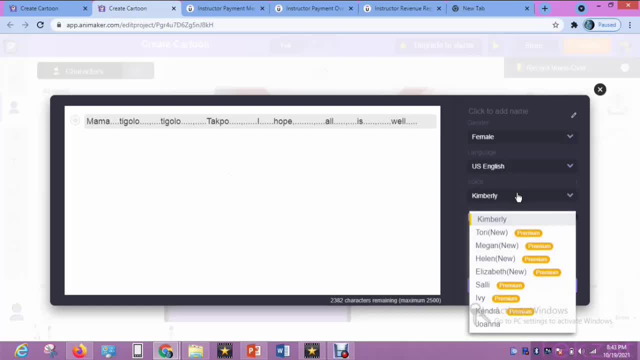 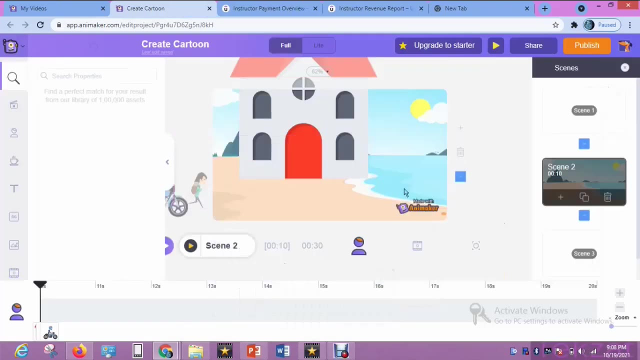 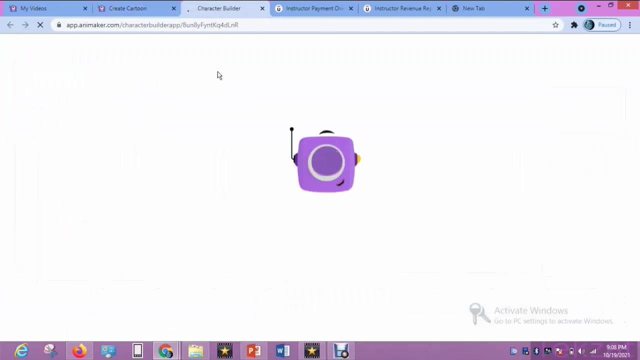 can change the language. We're using English here. Um, it's in Johanna, So let's listen to her. We're going to create our own character. This character: click here. Then click here. That's add character. Create your own character. Good, Now this page, this page, So let's go. 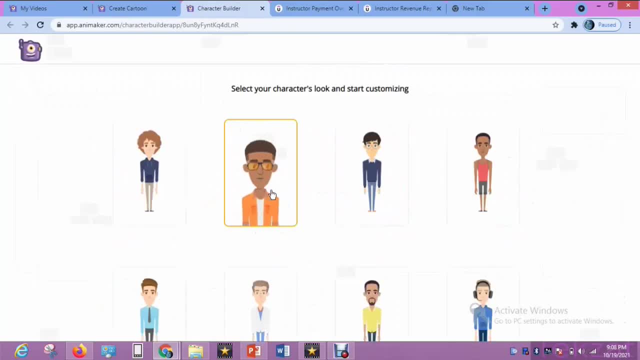 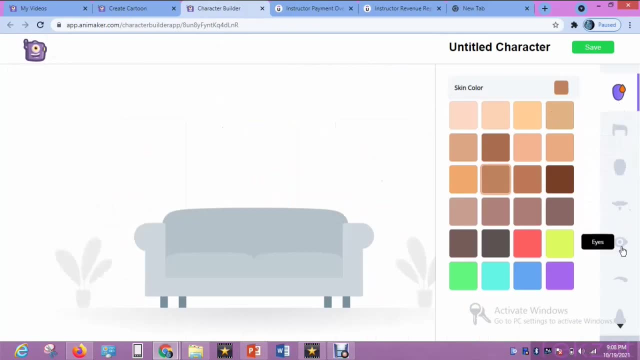 ahead and start from here. Uh, we choose this guy. I think that's ok. Let's uh, just follow all these instructions here. We're going to use the one after the other. Uh, we'll check here, But before that, you have to name it. I'm naming it Toy Toy, Toy Toy. Ok, That'll. 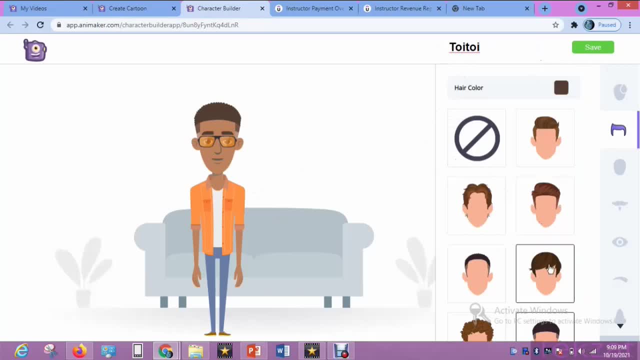 be the name. So we choose the hair. Um, ok, This hair will fit. see, Uh, that's cool, man, Bar head, That's ok. Check the face shape. Um, seems the talk is not friendly. Uh, we don't need. 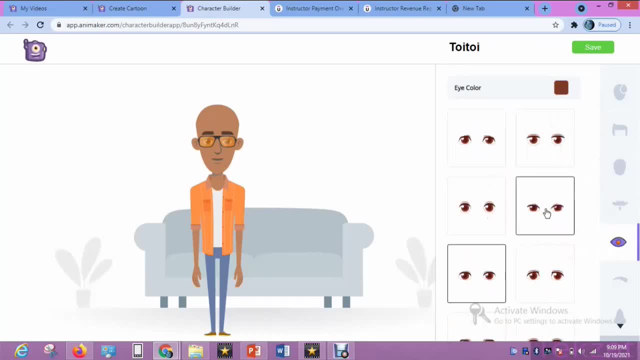 that, Uh, we check the eyes, We choose this guy. That's cool. Then click here to go down This nose, Eyebrow, This mouth, Love this. Um, this is ok already. Uh, so we'll click here to check other ones. This ear, Uh, choose any one, Ok, Frown Winkle. 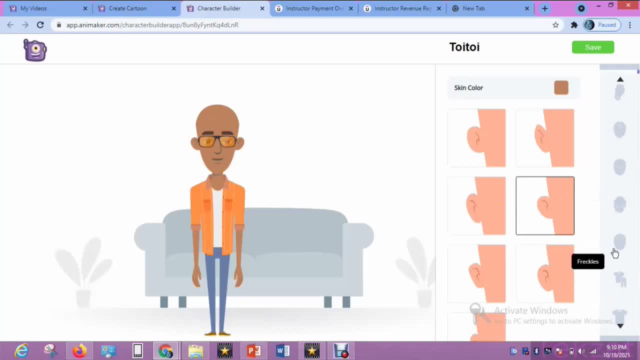 This smile. Ok, Ok, Smile, Smile. Then this shirt and trouser: Uh, we choose any one here. Let me go for this guy. Uh, that's cool, Uh, huh. Then you can also change top wear and bottom wear. Ok, So let me change bottom wear And. 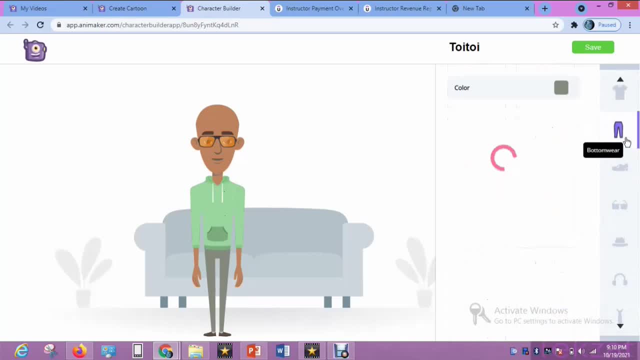 then Ok, Ok, Ok, Ok, Ok, Ok, Then I'll choose this guy. Uh, that's cool. So Spectacle, Wow, This beauty, Um, this fine, This fine, The guy, two different, eh, color Spectacles, That's fine man. 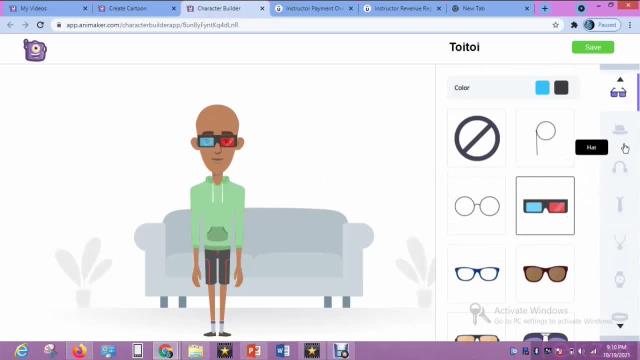 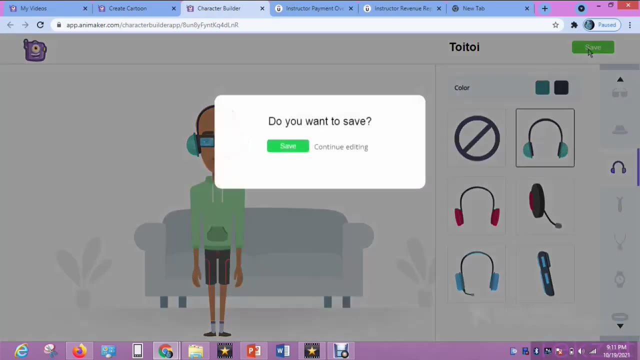 Uh, the other one Half-ass. Therefore, let's give this guy music man. The guy will like this 3.5.. that's cool, so let's save this. okay, now we're going to save it. yeah, the way for it to save. 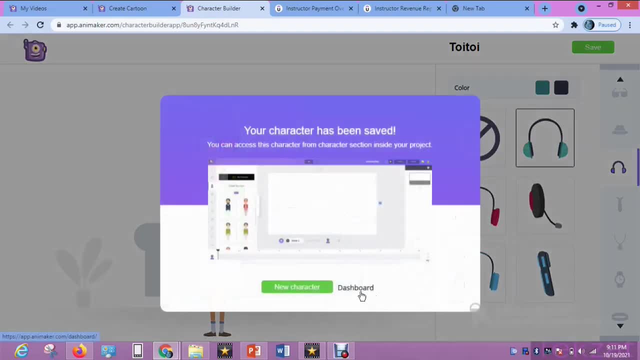 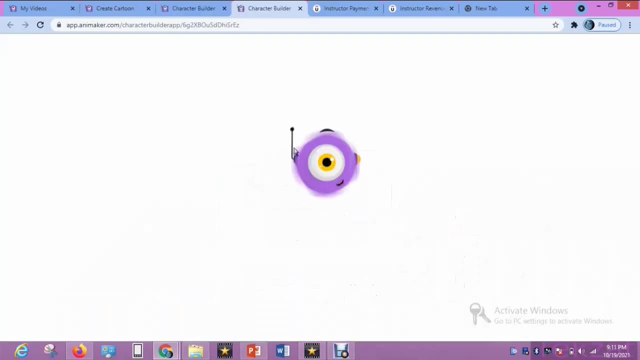 it takes time. good, yeah, saved, is that similar? so now we can go back to dashboard on new character. so we'll say: new character, I'm going to create another one. this time around we select female and then this lady will be fine, this girl, which one you prefer? this, this, this, this, this, this well, 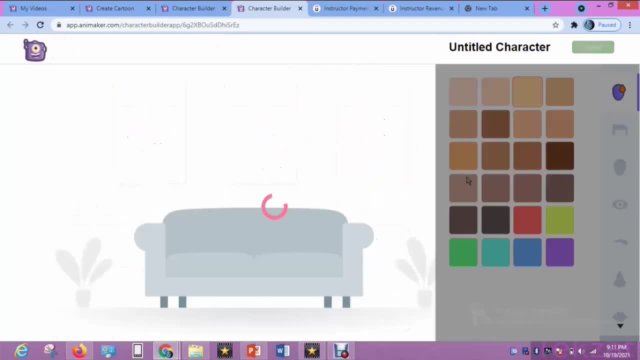 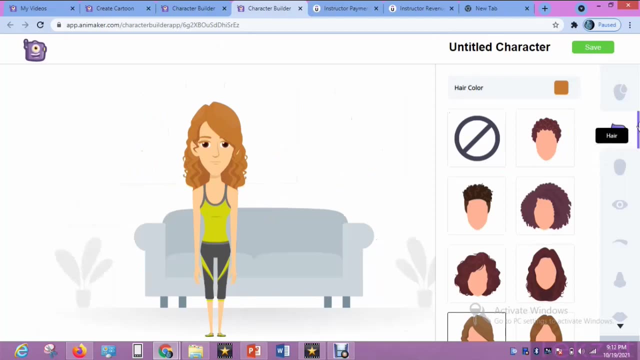 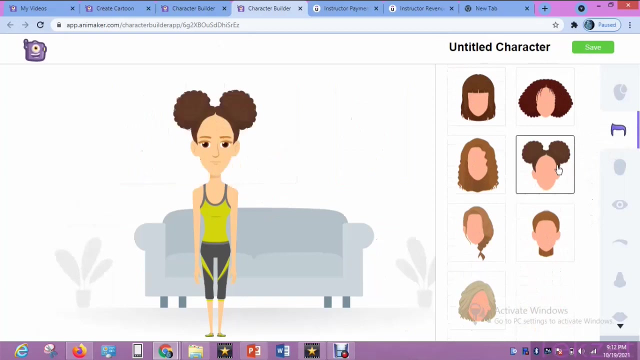 let's go for this, okay. what much to change here? let's see the hair. Wow, a lot of her stress. yeah, okay, this is okay. look like a small girl, yeah, oh. face shape: yeah, yeah, bro. oh my god, it's a special mama. yeah, go for this, this cool. 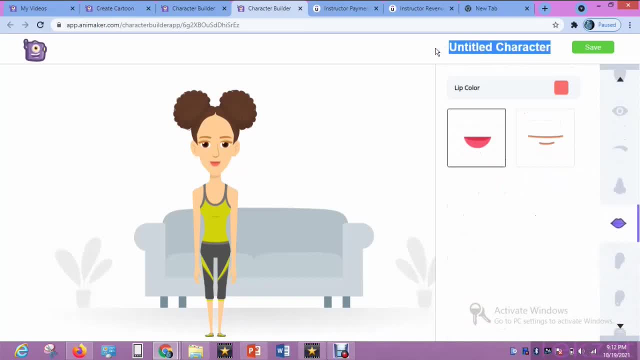 right, let it would never her hair, okay. so you tell us if your name is twingcuh- twingcuh- I don't know the meaning, so let's check another thing, okay, yeah, yeah, and she needs one. she needs saw which one will be better. 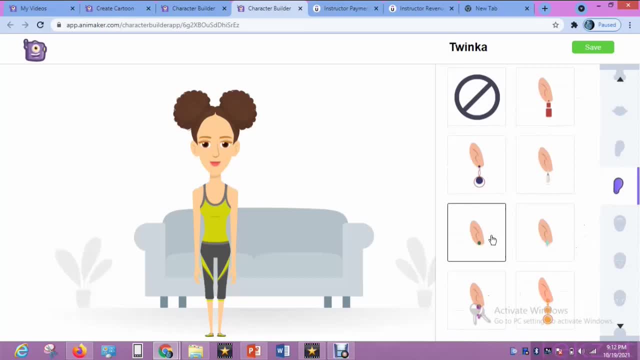 that's what I'm saying. your name is nothing like this, nothing again. let's see this one: wow, she's just fine. okay, and one again. you are good for top, okay, oh, that's it. uh, this one is: wow, that is great, that's great, but that way. 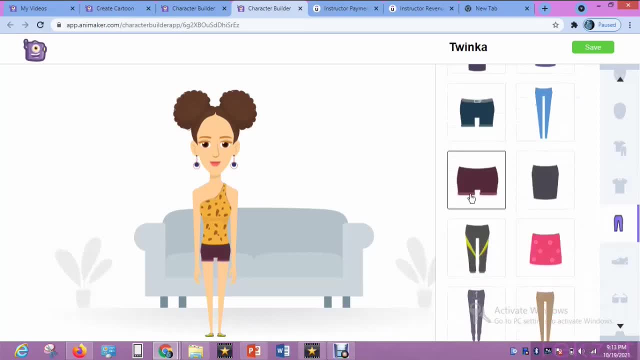 okay, how about this? no, that's too short to me. okay, let's check another one like this will match it. yeah, i think this is okay. uh, whatever, i'll give the guest spec. no, because i don't like the guy where he's fighting everywhere and this will be fine, yeah. 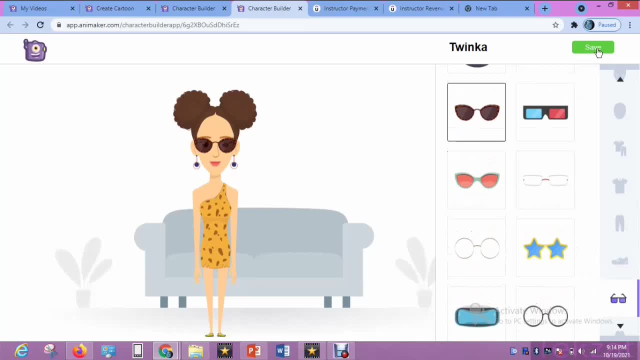 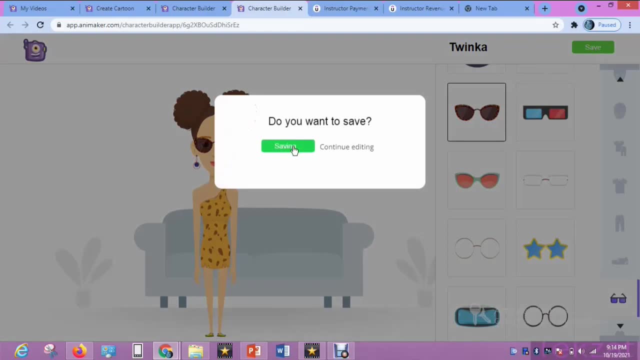 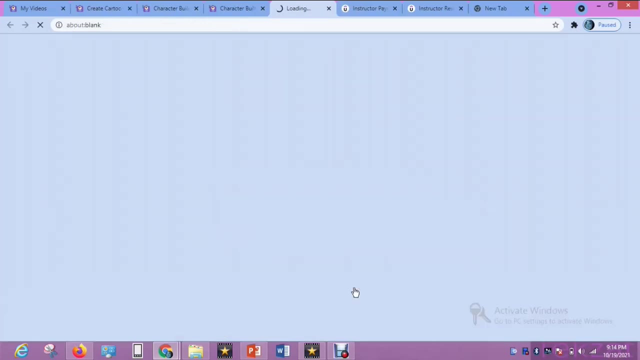 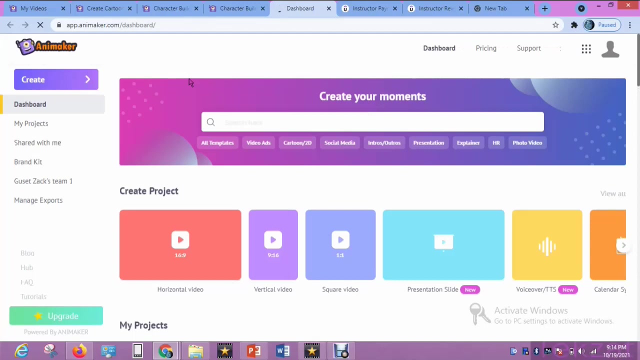 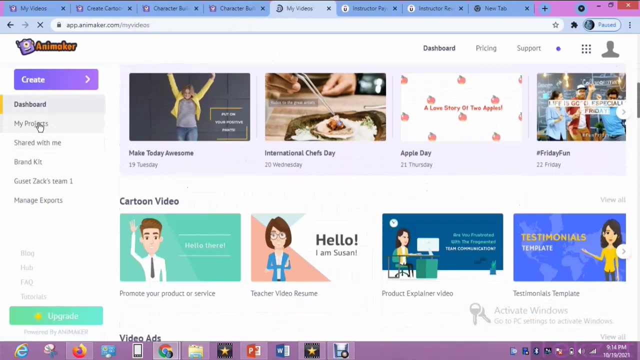 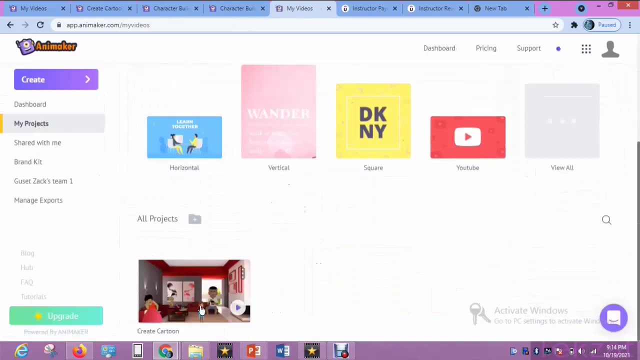 a beautiful twinker twinker. that is okay, so i've saved it. so go to dashboards. remember we just created two characters, so that how characters have been created in this kind of uh platform. so these are dashboards. check out the process again: what projects, projects? and come here. 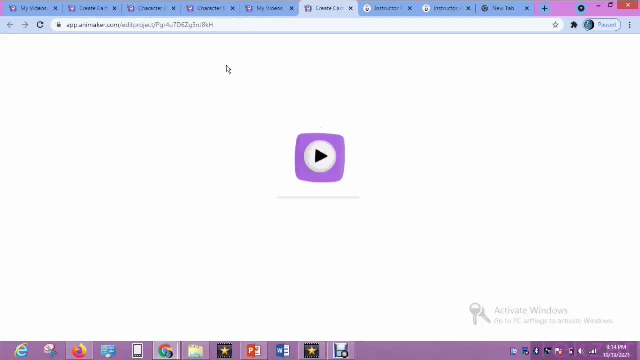 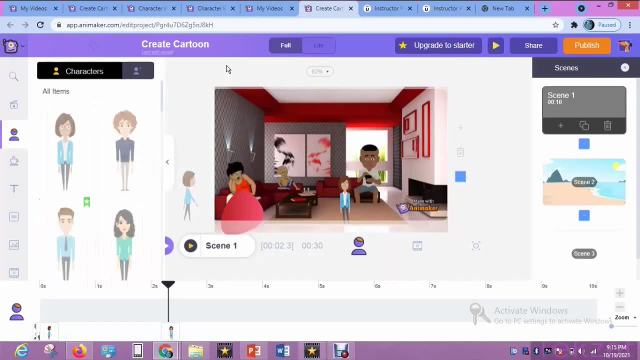 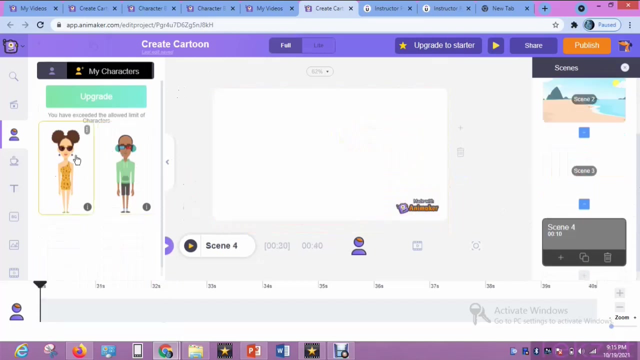 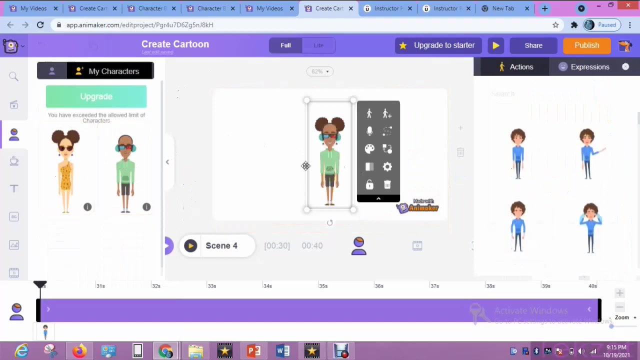 too many many projects. okay, now look for a karata, a special karata. ah good, these are two karata. you have a city limit of karata, okay, so now let's create another scene, create new scene, then load our karata. one and two. good, okay, these are two karata, and 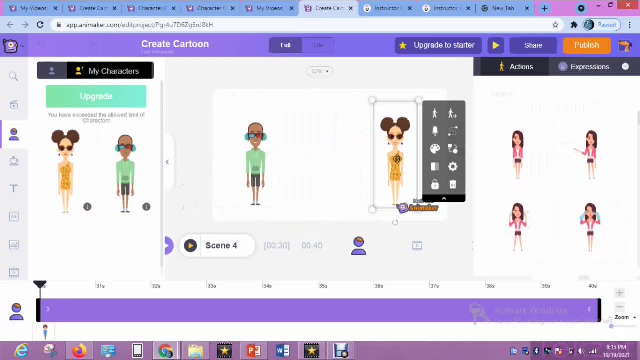 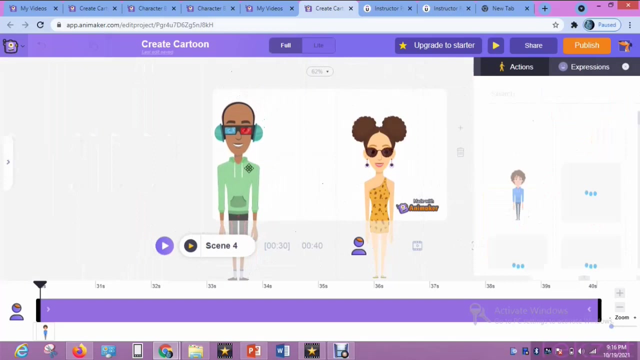 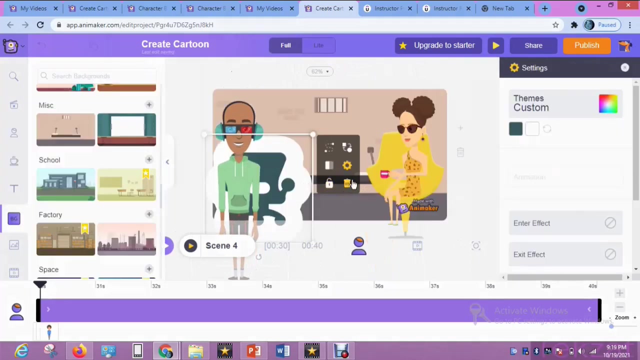 the next thing they will be discussing, telling us what we know about the slides, this karata we just created and let's increase it. but then look, little bit bigger, the bigger seems this workspace is too small. okay, good, so now working with these two karatas and give the transparent going off. that's it. 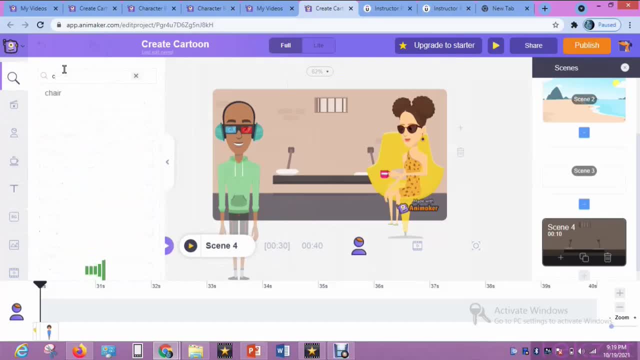 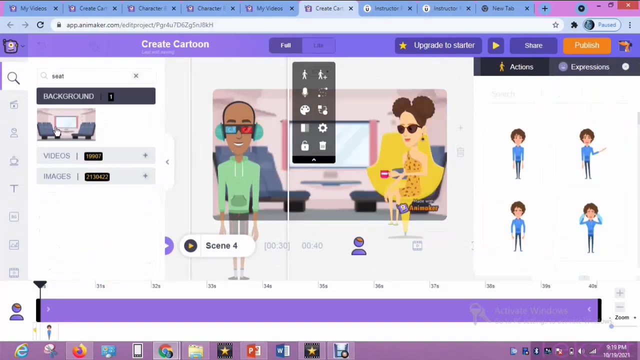 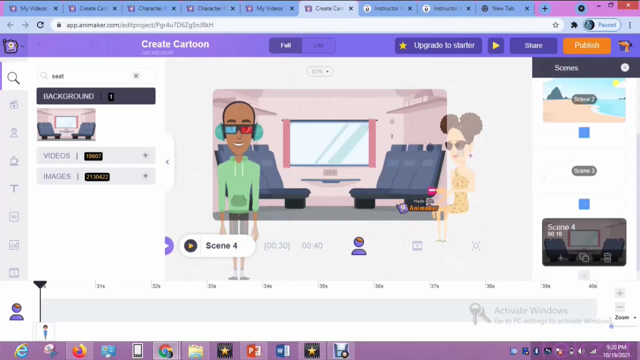 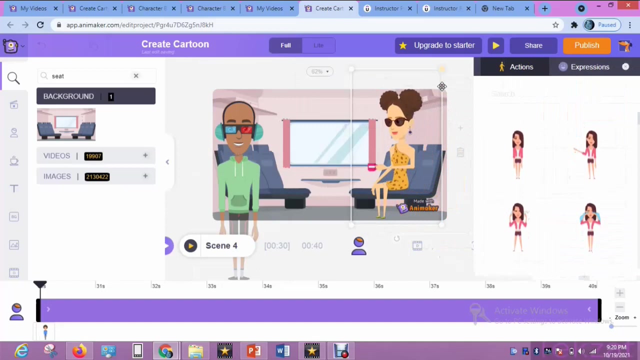 all I just see. let me see, hmmm, I need to switch sides. I look for, okay, well, this sounds like this will be better. yeah, oh, that's cool, that's cool, that's cool. so this background has city origin. mhm, yeah, mhm, wow, and this guy here will also sit.